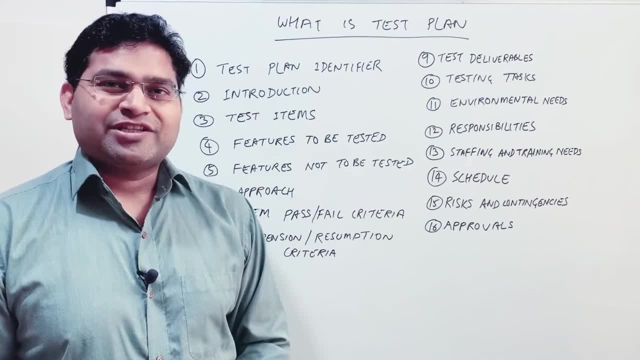 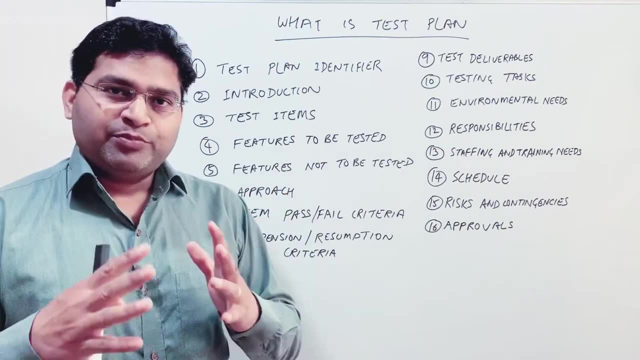 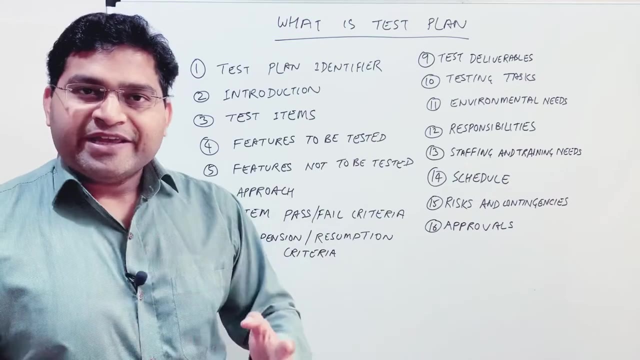 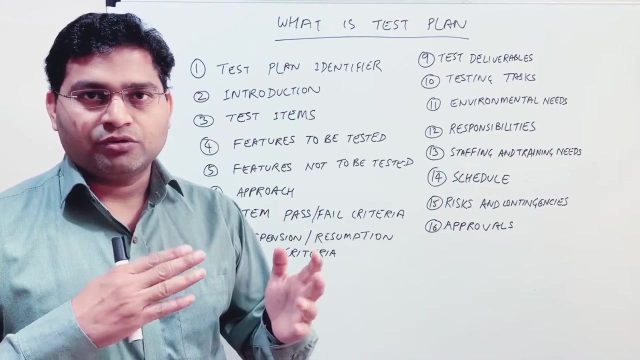 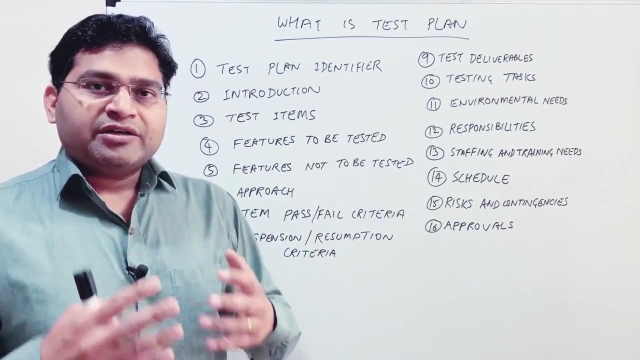 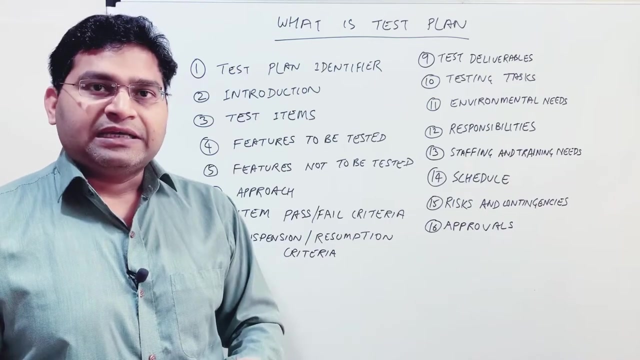 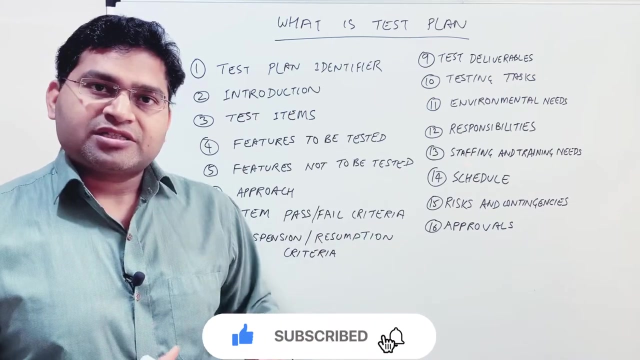 Hello everyone, welcome again. In this software testing tutorial we are going to learn about what is test plan. Now, before we understand what exactly is test plan, I'll explain in general why planning is important and what a plan is. Now I'll take an example of, say, you know you are building your house, So you have bought the land and you are building the house. Before building the house, there are a lot of planning activities that in general happen right. So you have the you know floor plan made and then, based on that floor plan, there are other planning that needs to happen before you actually start putting the slab and then putting bricks and building the walls right. 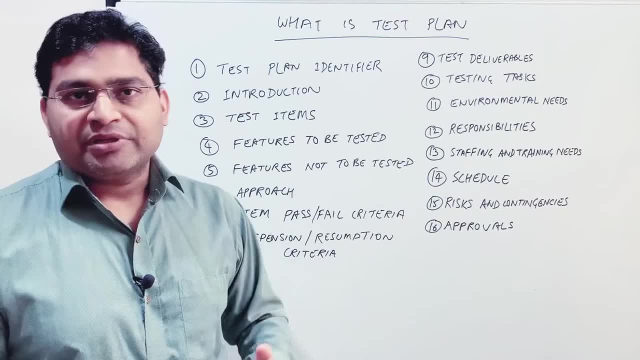 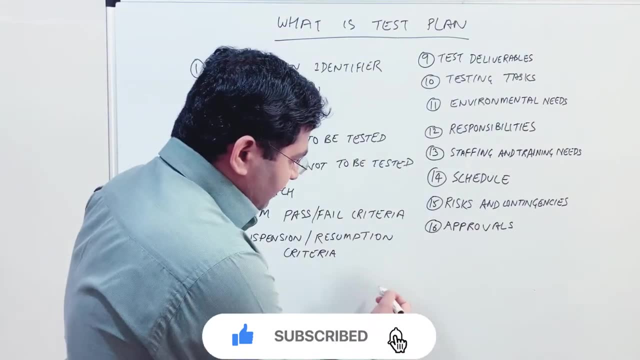 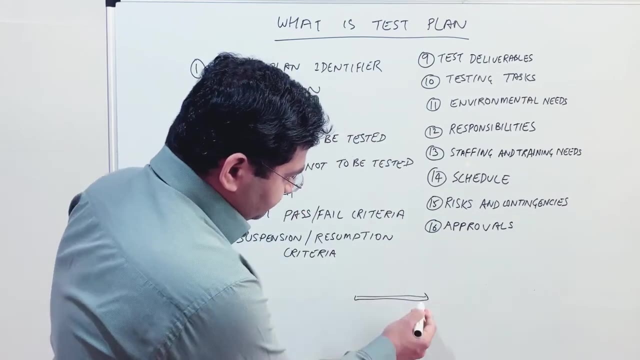 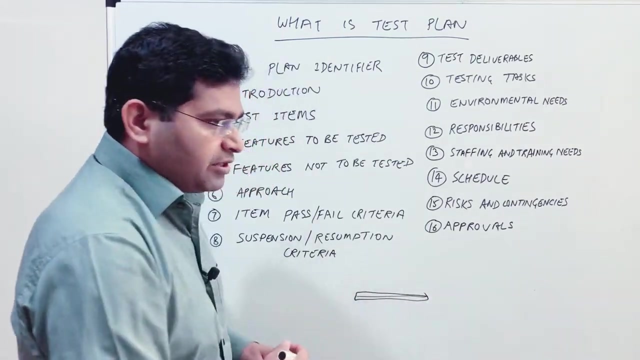 So what is test plan? Why does it happen that when you are building the house, you plan it first? The reason is say, for example, you are, you know, having a piece of land and say, for example, you start building the slab altogether. okay, So you have laid down the slab on the overall area and after that you realize that you forgot the plumbing work. okay, So plumbing needs to go beneath your house and it needs to be. 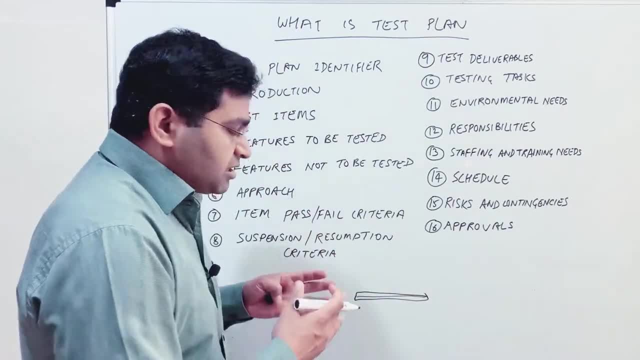 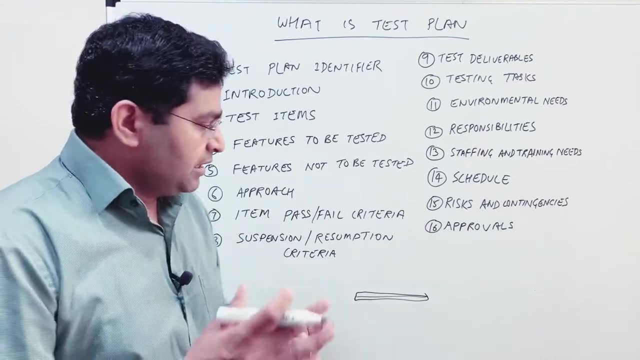 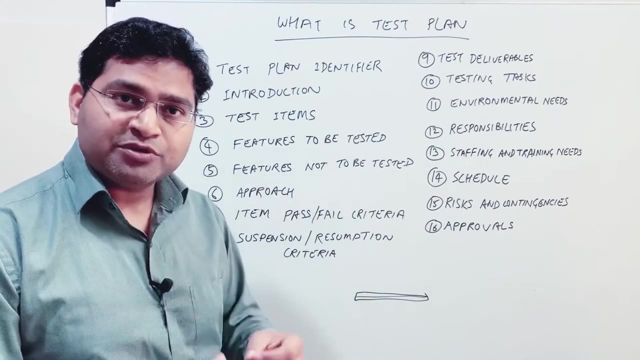 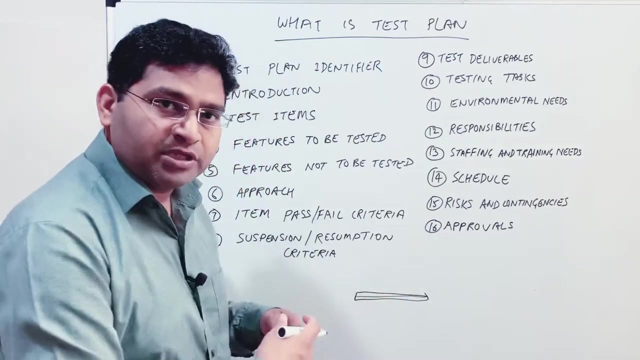 planned properly. So these are some of the issues that happen if you do not plan your work properly. So planning in general is very important. So when we build the house, we build the plan and plan covers all the you know small things and it helps you to basically give a bit of you know thought what all needs to go there. There needs to be plumbing, there needs to be electrical work, how electrical work will happen, where based on you know, like the floor plan, etc. 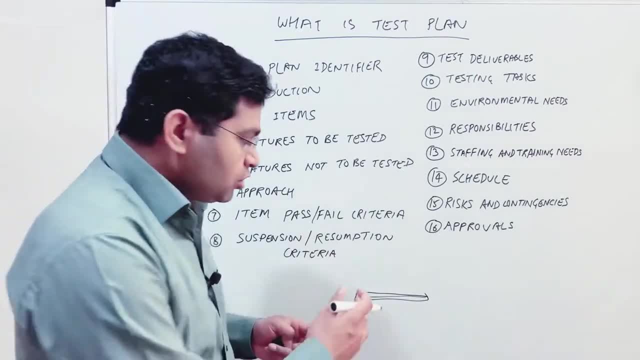 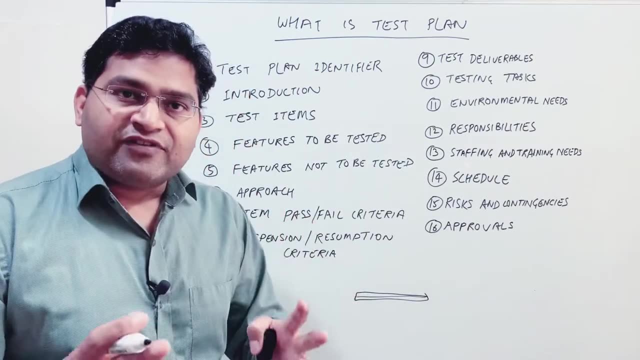 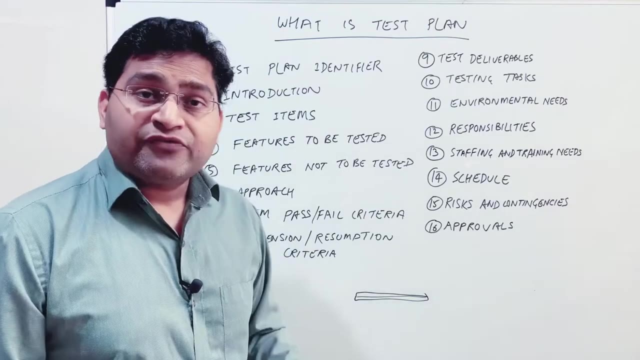 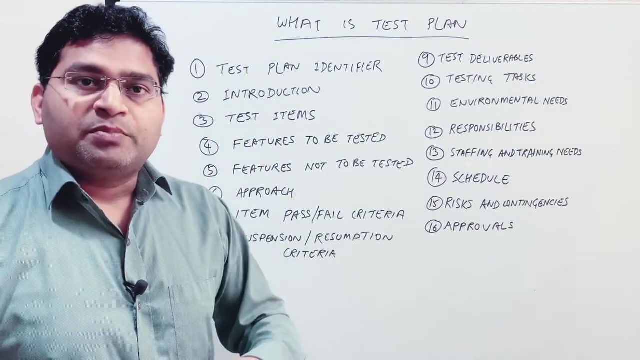 Where the bathroom will be, where the kitchen will be, what all plumbing and electrical- you know- connections need to go in each of those rooms. That all is defined in your normal house plan. right Now, when we talk about the test plan, it is no different with any other planning activity. So when you are building the house, you build a plan to build the house. When you are doing software testing, you build or you create a plan to build the house. 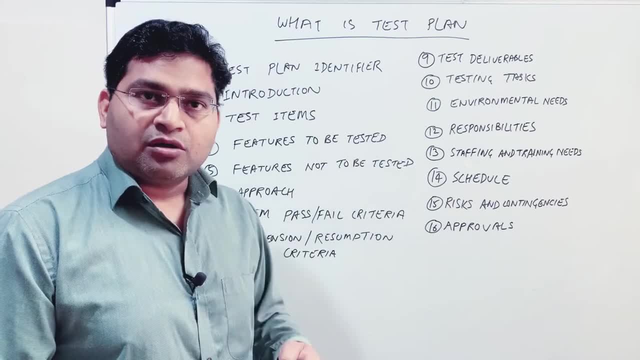 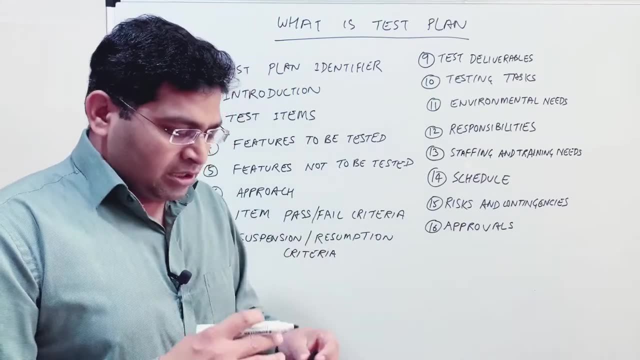 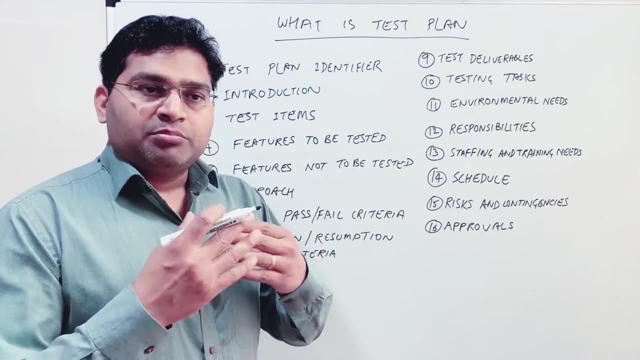 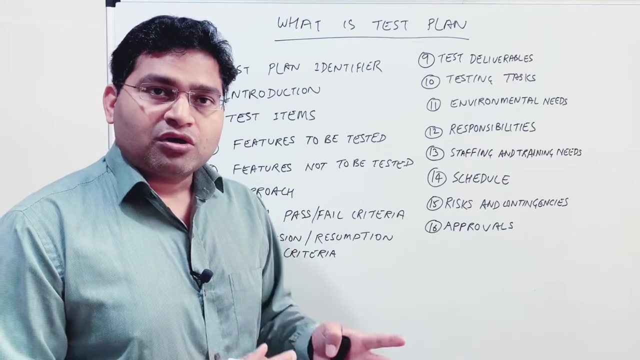 To basically mention or identify what and how you are going to test a particular software, right? So planning gives you a predefined or gives you a guidance to basically analyze what you are going to test and how you are going to test. okay, So there are a lot of you know templates available and the you know organizations. 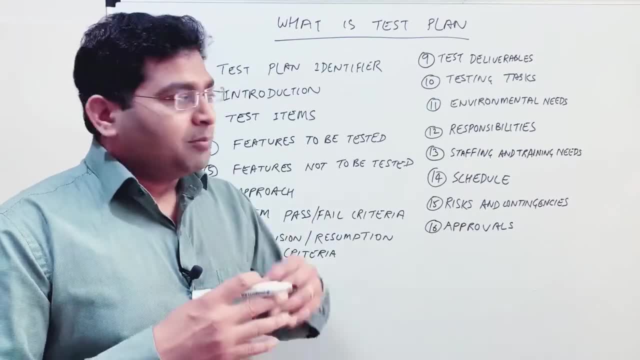 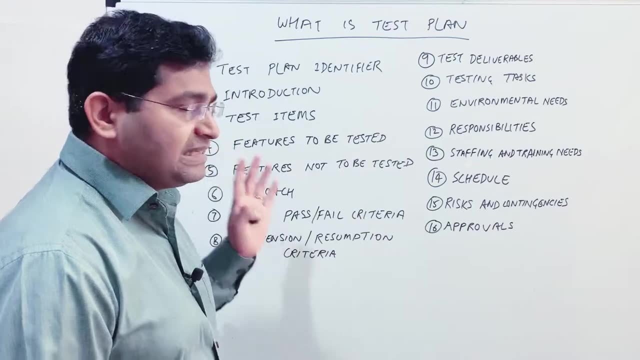 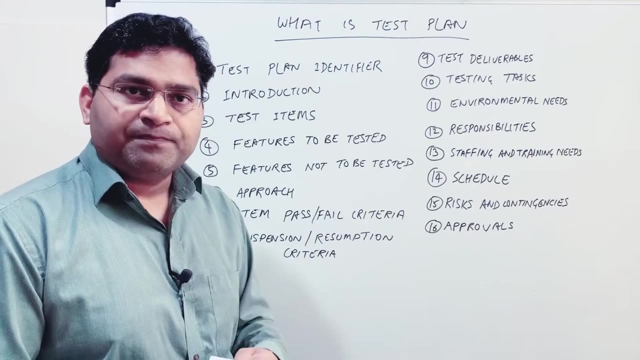 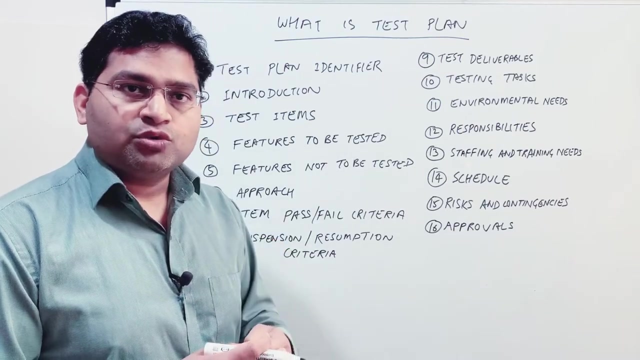 you can customize these templates accordingly, So as per their needs. But in general, test plan template, this is IEEE template sections. These are the key sections that need to be included in the test plan. So we have understood about the general plan and planning. So planning is important. Without planning, if you start, you know actually doing some work, you are, you know, going to end up in some sort of trouble or you know you might have to do some work. 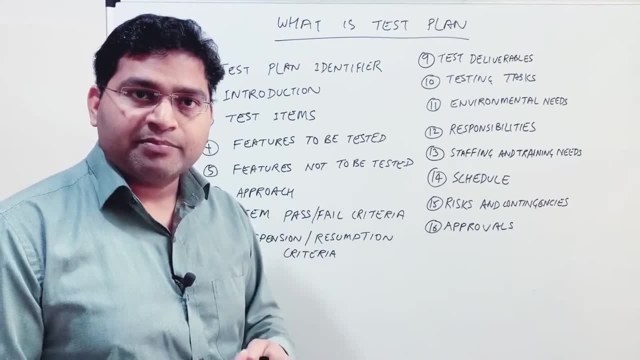 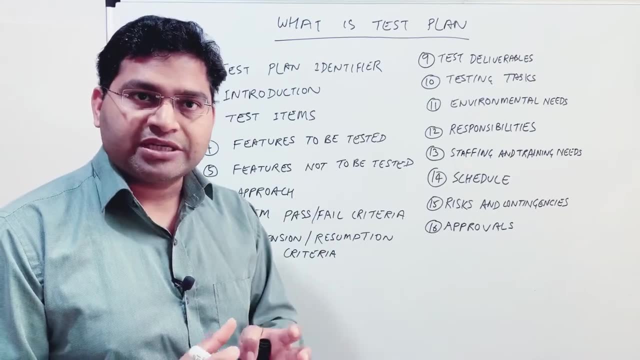 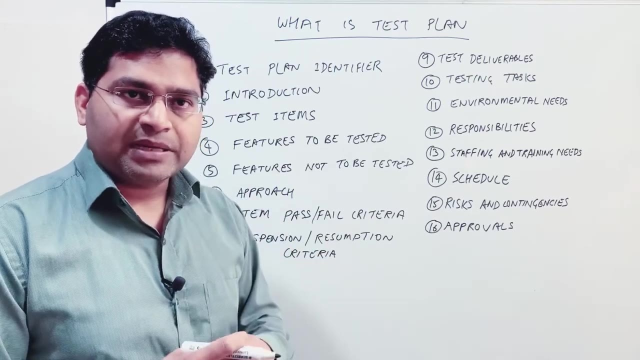 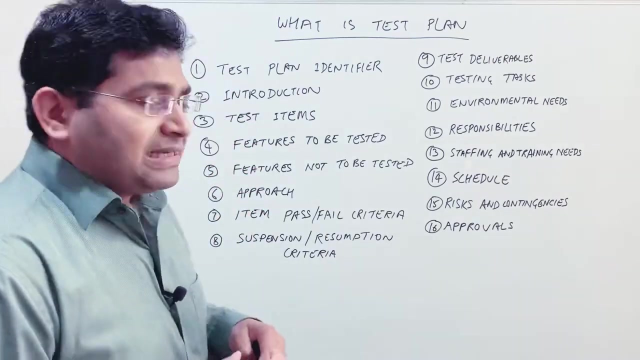 You might be forgetting something, But if you have, you know, proper plan in place, then you give it a thought about the software testing module that you are going to test or the overall software that you are going to test And based on that you know testing or the thought that you have given in that particular plan, you define all the activities that need to go in that plan, step by step, right. So if we talk about the test plan, you know what all needs to go into the test plan. 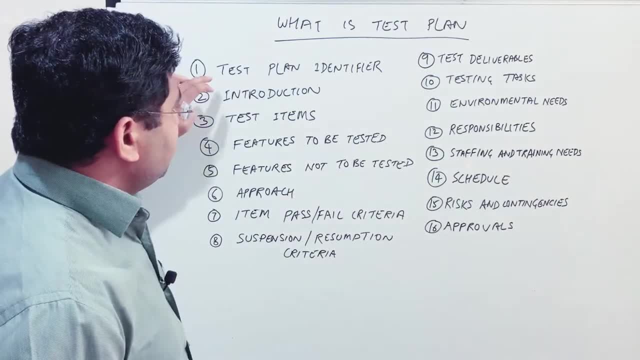 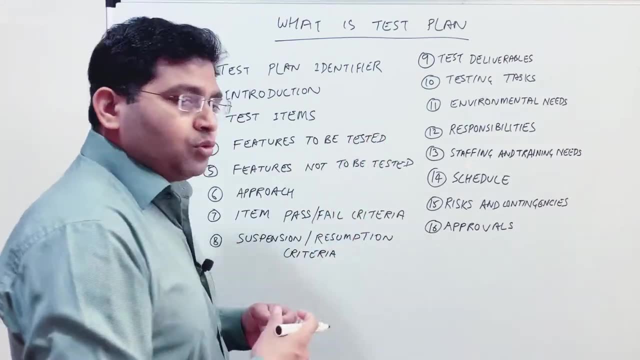 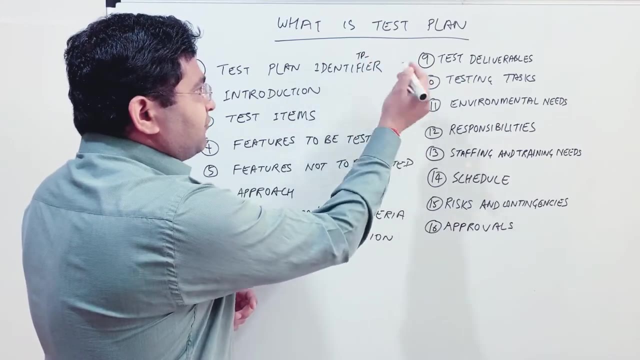 to software testing and in the test plan we have, the first thing is test plan identifier. now, when we talk about test plan identifier, it is something you know, a document identifier. say, for example, you write something you know, TP underscore, and then say, for example, your project name or initials are ABC and 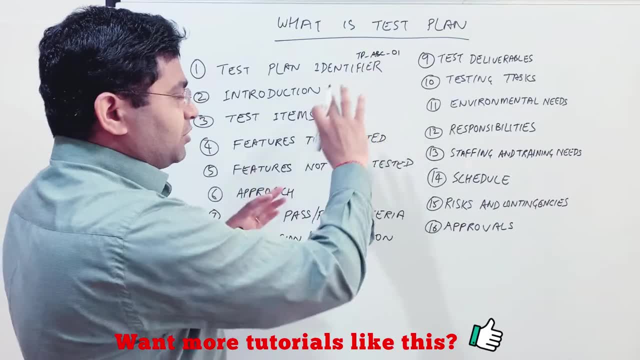 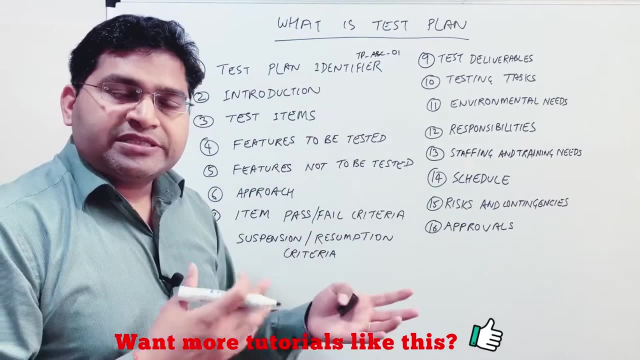 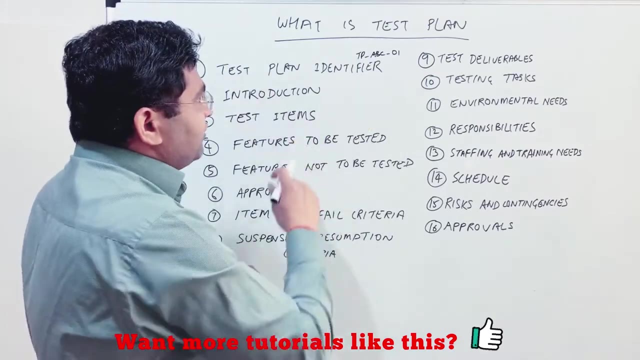 then you start: you know 01 or something, so this is something you know you. you basically provide the name of the plan so that anybody who is seeing can easily understand that this is test plan of this particular project in the organization, right? so test plan identifier is identifier of that. 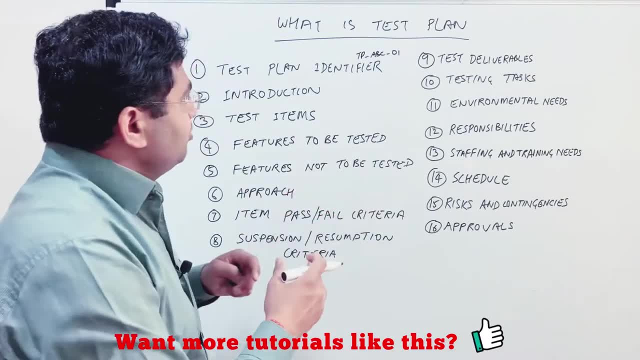 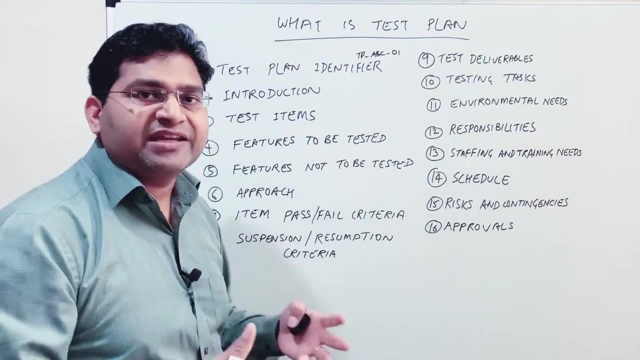 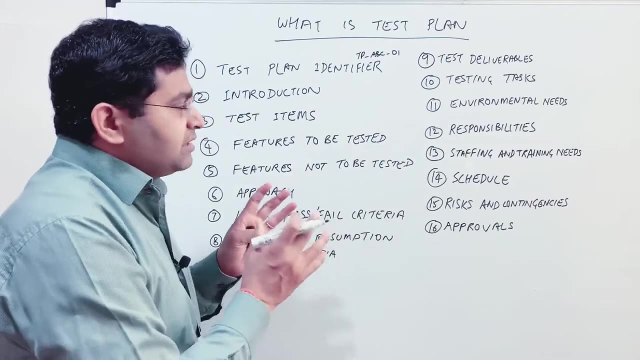 particular document that you'll be creating as part of the project. then, in the introduction section, as the name suggests, you will introduce what this plan is all about. right, so which particular module or which particular application, this particular test plan that the document that you will be writing will. 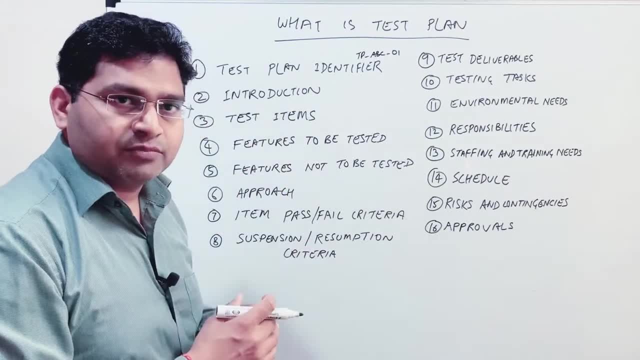 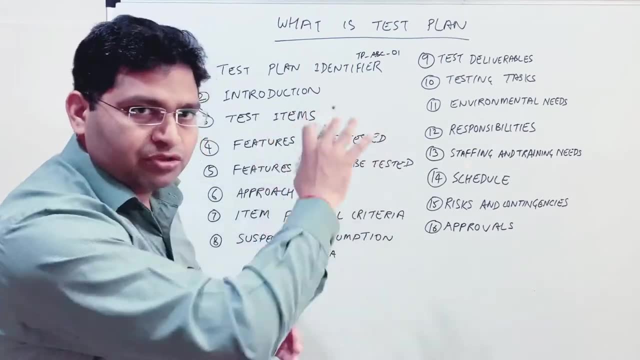 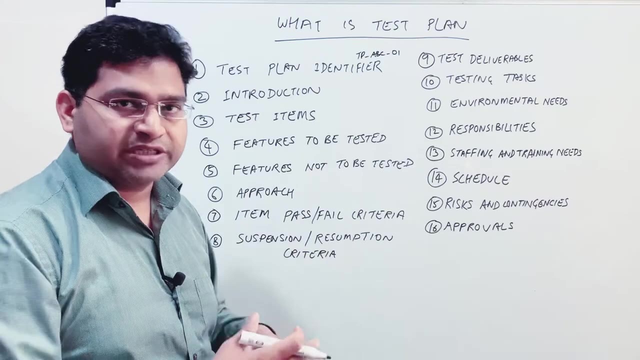 be you know handling or we'll be testing for. so introduction about the project and some of the details about the project. so couple of you know statements there in the introduction section so that if anybody reads that introduction section he can or he or she can understand what exactly the plan is all. 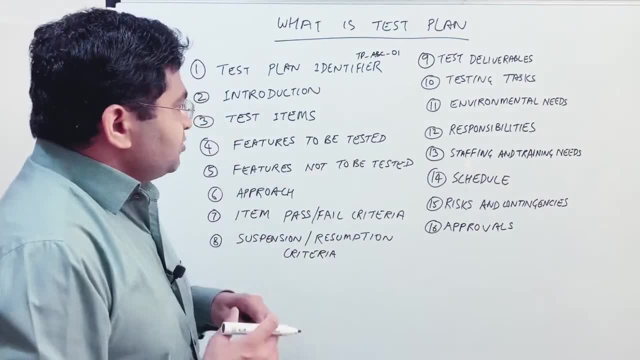 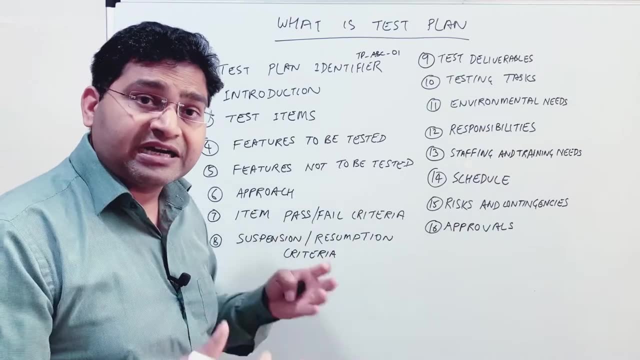 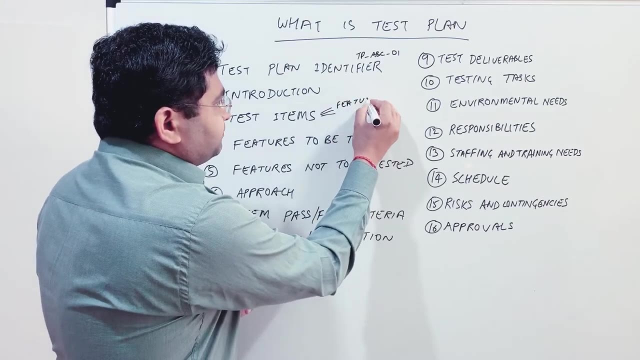 about. okay, then you have the test item, so this is another important thing. so what this will guide you to you is, when you identify the items, or the testing items, what this means is all the features that you are going to test. right, so high-level, you know features, or? 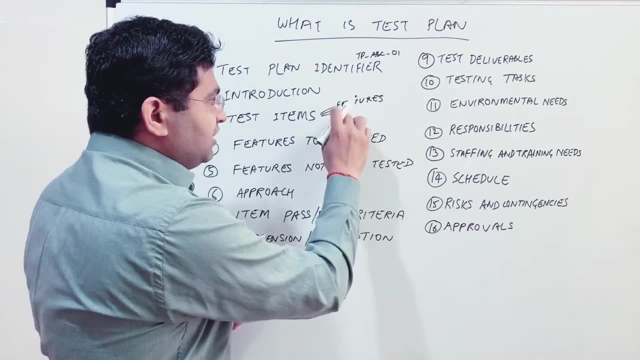 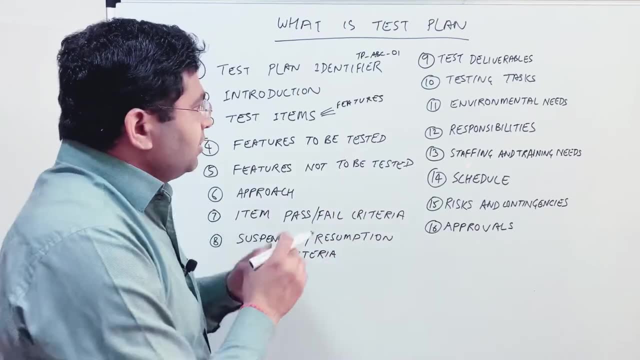 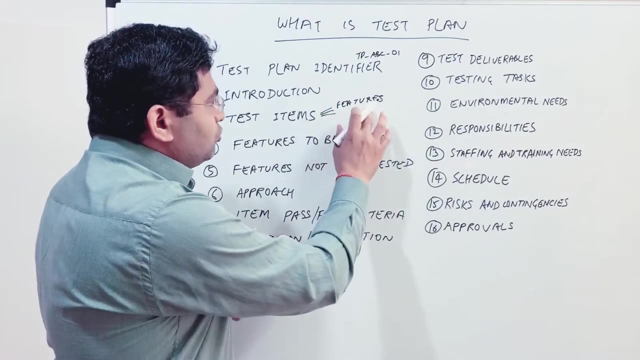 the requirements, right. so if you have the requirements or the features, so there'll be. you know, like high-level features say, for example, if I am testing a e-commerce website, then what all features need to be built as part of the release one or release two and then you include those feature. so, for example, 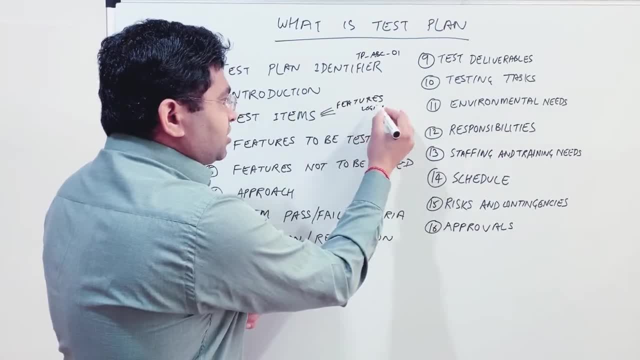 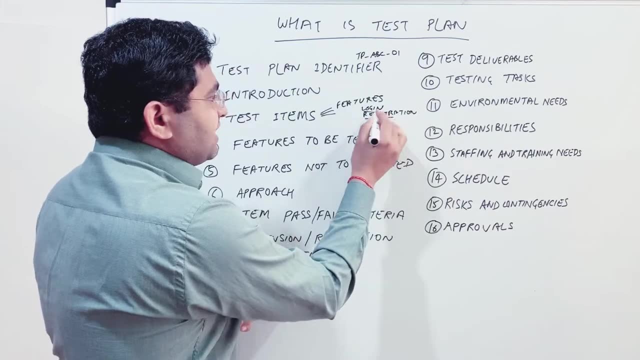 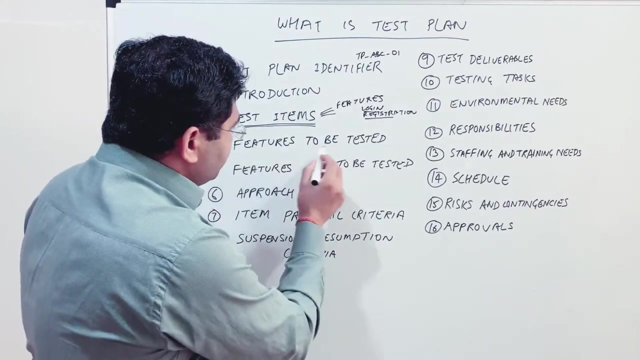 login functionality. so you mentioned login with some of the details. then you mentioned registration. so high-level, you know functionality is that you are going to test as part of the application. you provide those details in the test item section of the plan, then you have the features to be tested and features not. 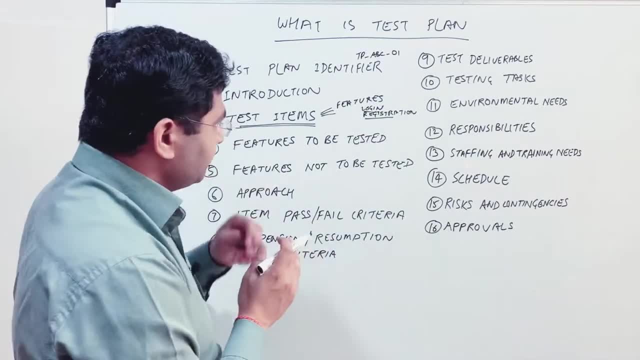 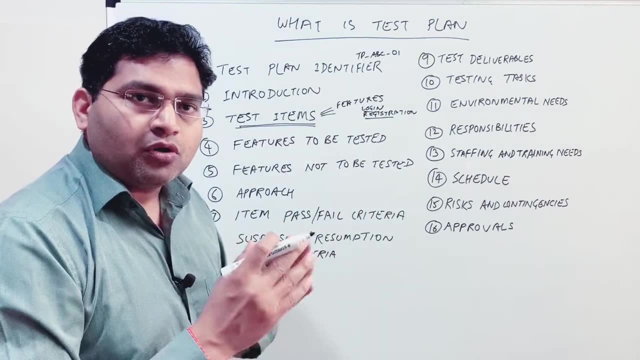 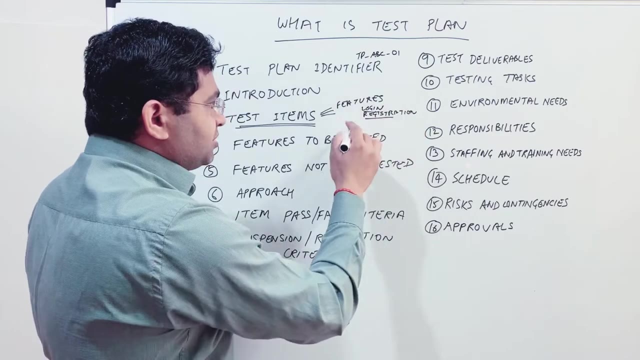 to be tested. these two are also very important sections of the plan, and in features to be tested and features to tested, then you can see the first one, which is the tested you mentioned, or you, you know, write down all the features that need to be tested. so, for example, here we have already included the test items as such. 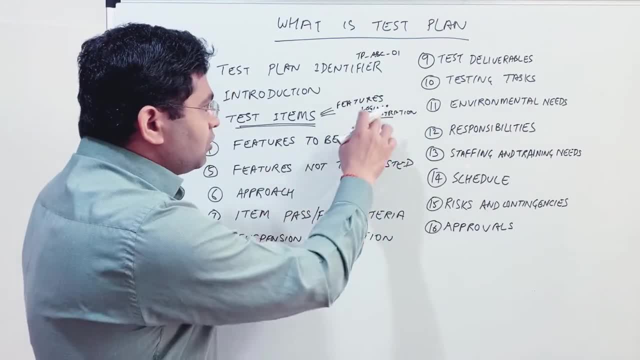 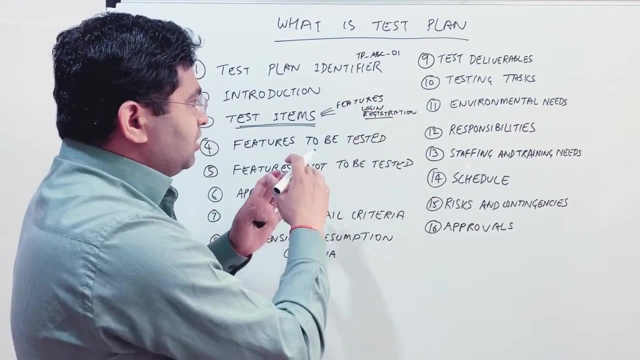 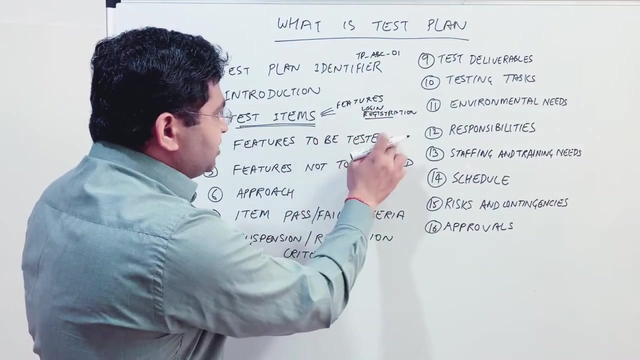 now we have to basically elaborate what all features of these items, right? so in this case, say, for example, you know test items are login or registration or any of the detail. so what? all features among those items need to be tested. okay, so whatever items you are mentioning here at the test item level, then you 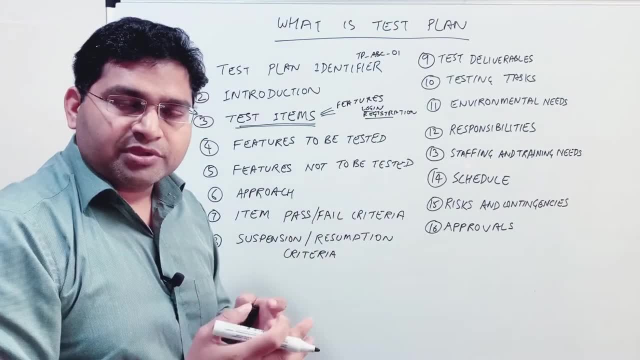 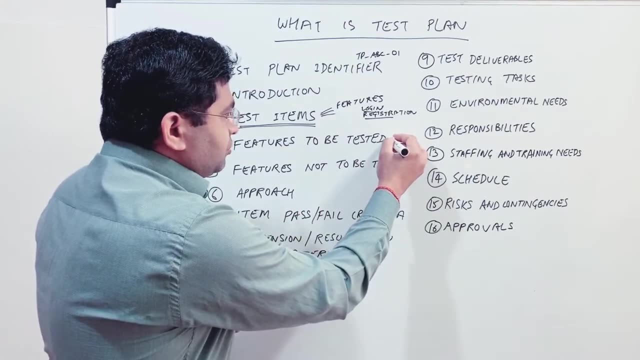 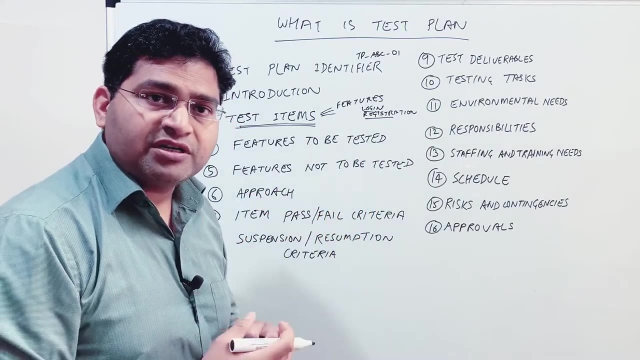 elaborate what all features within those items or high-level modules that you have mentioned here in the test items need to be tested here, right? so those all details will go into features to be tested then. features not to be tested is also very important because you need to upfront analyze what you are going. 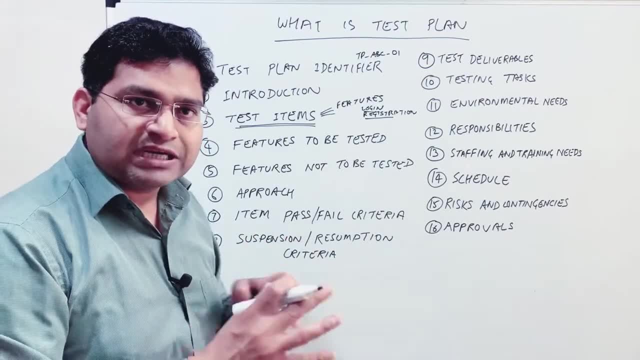 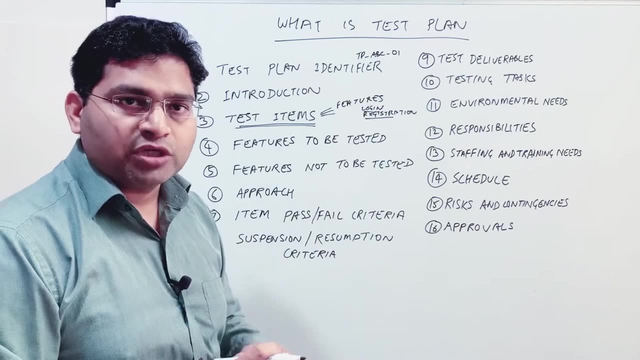 going to test and what you are not going to test, right? so this gives you a clarity that when you are starting to execution phase, then you know what you are going to execute and what is basically required as part of the test execution, right? so you mentioned whatever features need to be tested. 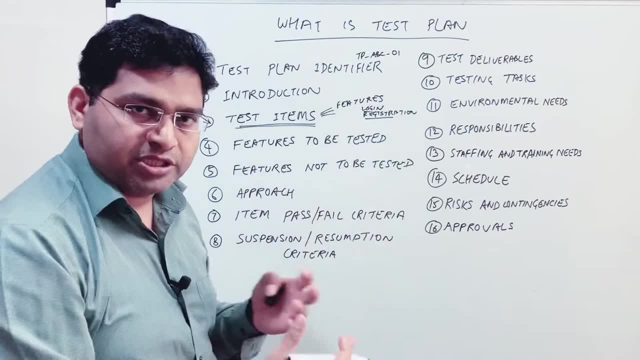 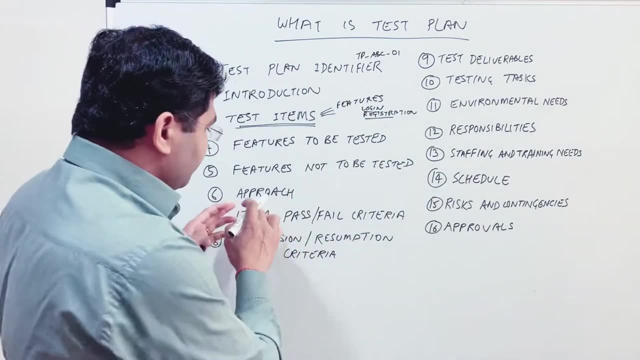 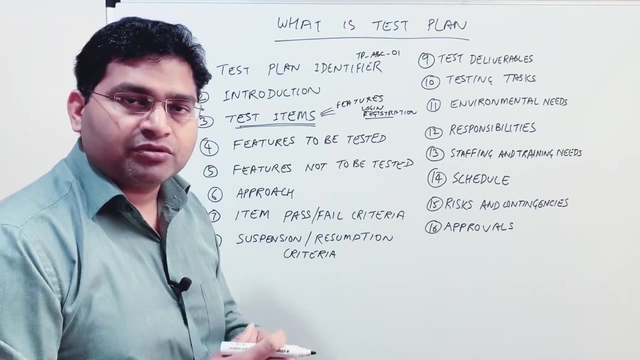 in the features to be tested, features not to be tested in the features not to be tested section. then the approach is another very important section and you will spend a lot of time on approach because approach changes based on the type of- you know- application or project. that 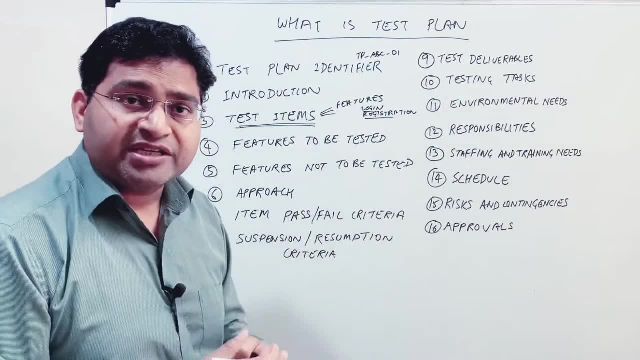 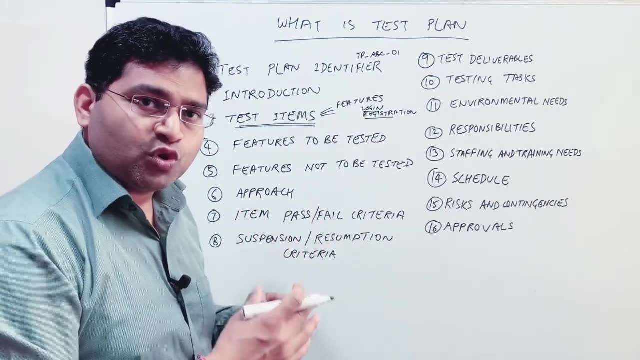 you are working in right. so, for example, you are testing a banking application, the approach will be different. and if you are testing an e-commerce application, approach will be different. and in approach, what mainly goes is how you are going to test a particular application, what all interfaces. 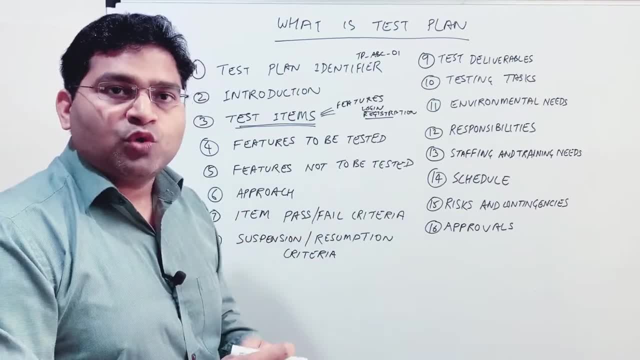 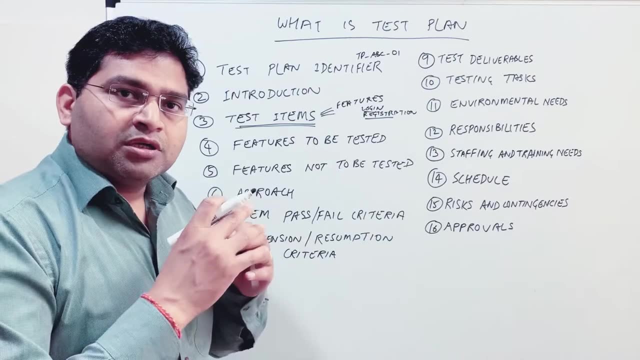 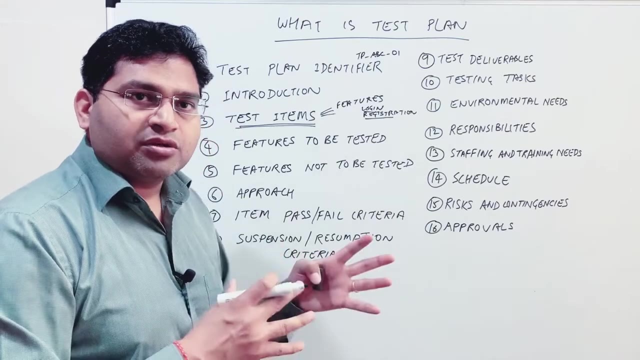 are there, what techniques you are going to apply, what will be the test levels, etc. so all those details go into approach, right? so you have to think about the particular you know product or application and then, based on that particular application or product, you define the approach or test approach for that particular application. 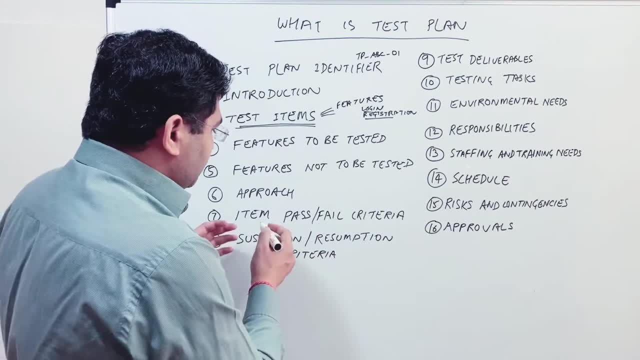 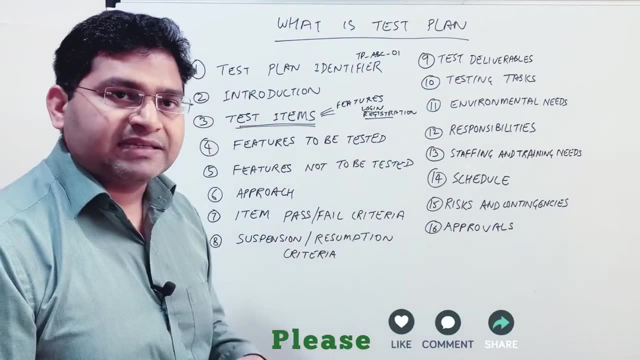 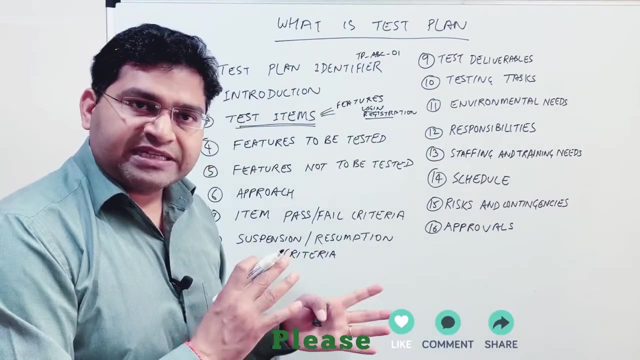 then you have item pass and fail criteria. so when an item will be considered, or the or a particular module or you know feature will be considered as pass or fail. say, for example, I have a module or a feature which has 15 test cases and when all those 15 test cases are executed, there are two test cases. 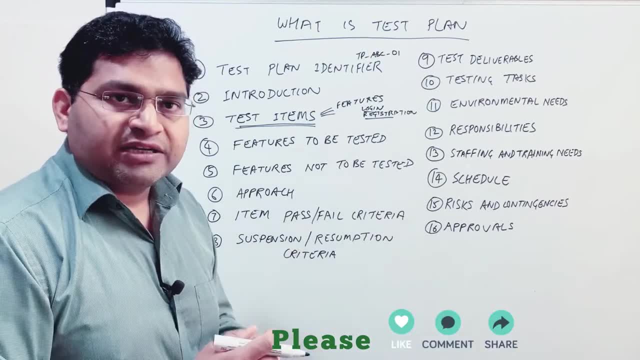 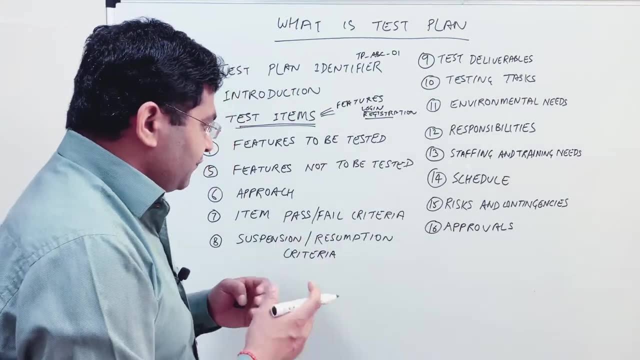 failing, which have low priority defects, still attached to it right or still open, then in the item pass and fail criteria, define where, what are the criterias which mark the item as pass or fail. so in the pass criteria you can, you know, make a decision based on the criteria that you have selected, and then you can. 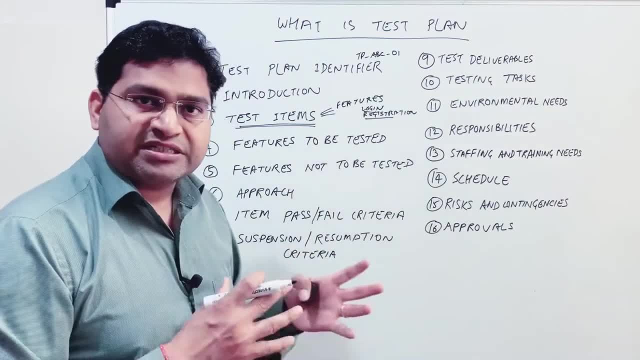 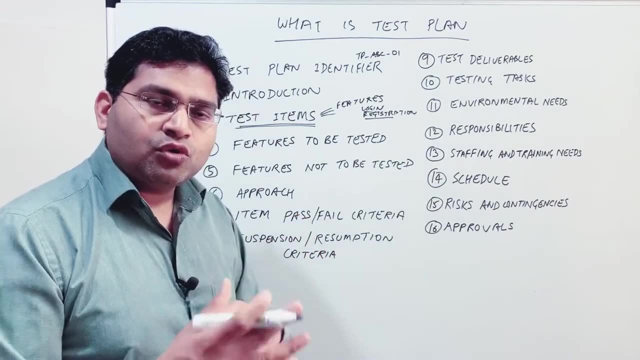 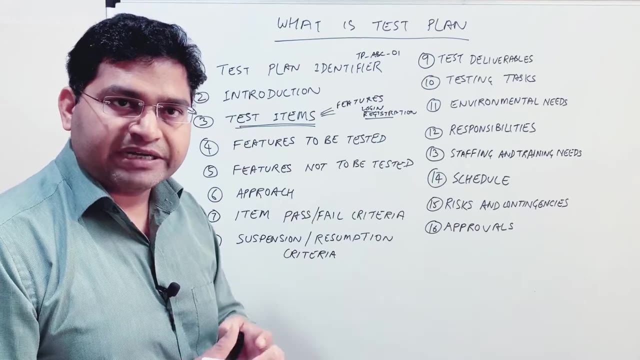 mention that and this is all. you know this as per discussion with the stakeholders or the members of the team. so in the item pass criteria you can mention that you know no severity one and two defects open, even if there are, you know, low priority or low severity defects still open if they are accepted. 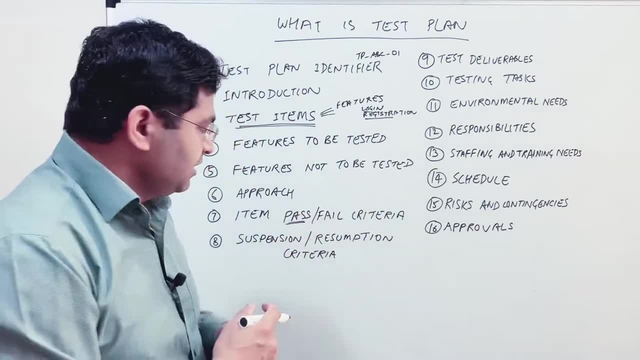 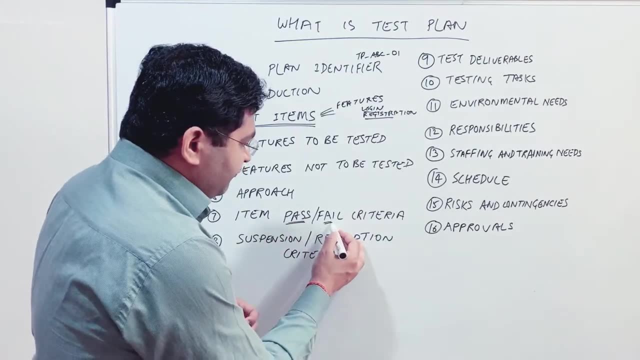 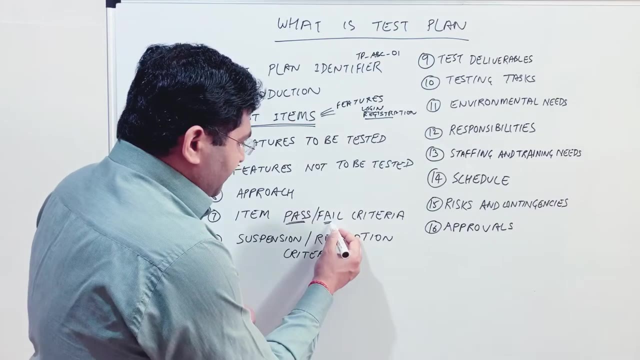 we can still mark the item as pass, right? so these are some of the statements that need to go into item pass and fail criteria. when we say item fail, you can say if there is any- you know, severity one defect or severity two defect, that is, you know, identified for a particular feature. then 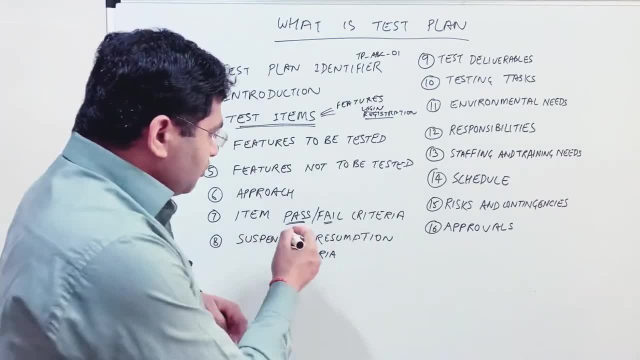 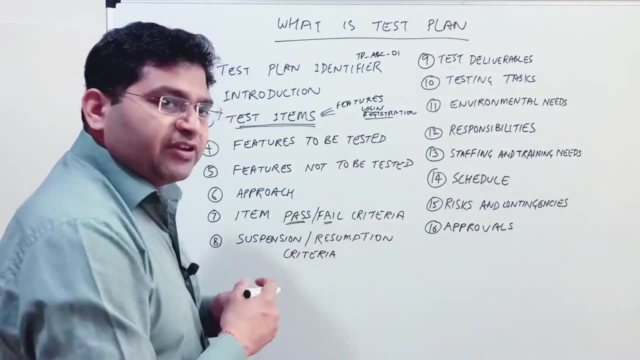 that is failed or that test case is failed. so any pass or fail criterias that can be defined need to go into item pass and fail criteria. then you have some suspension and resumption criteria. so suspension, as the name suggests. when will you suspend the testing right? 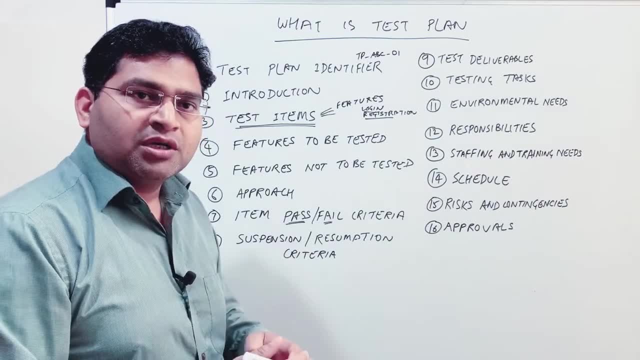 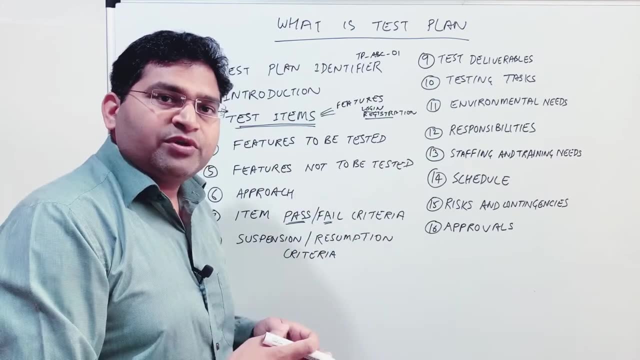 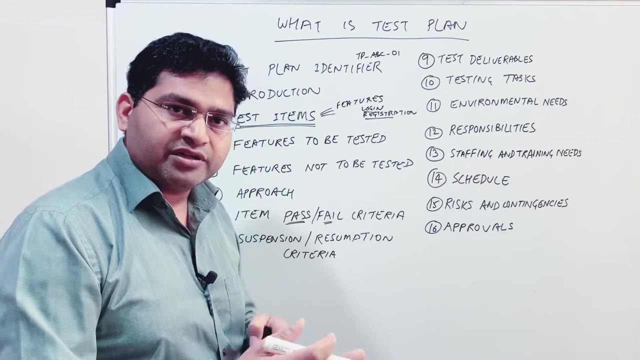 So suspension, as the name suggests. when you will you suspend the testing? right? say, for example, you got a blocker defect and the testing cannot progress further. or you got a defect which needs to be fixed, because unless and until that defect is fixed, all the testing that is done in future or further it doesn't make any sense. so in that case you will suspend. 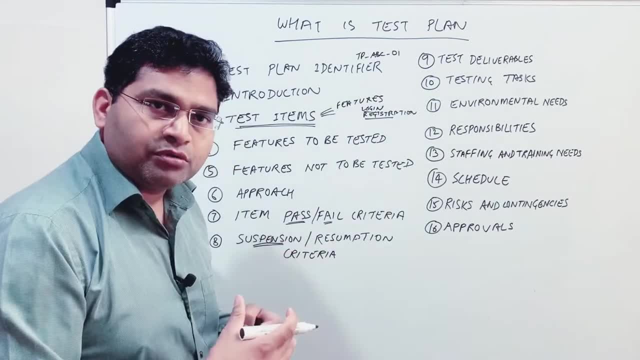 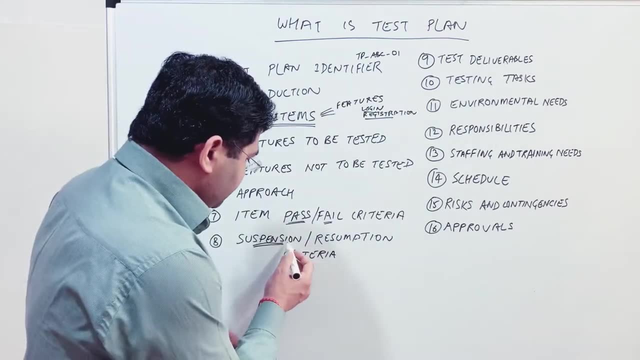 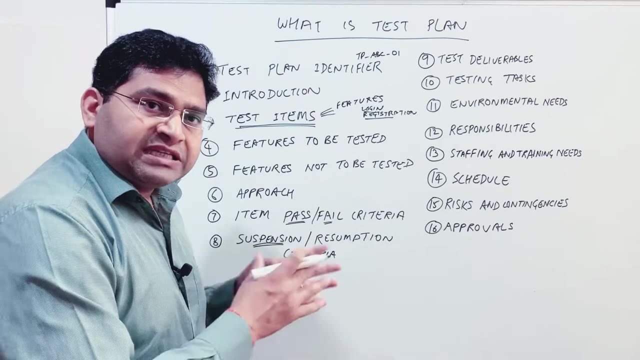 the testing. so any criterias that need to be, you know, identified and discussed with the team which will block the testing, need to go into the suspension section, and resumption is when you are going to resume. say, for example, testing got blocked because of these and these defects once. 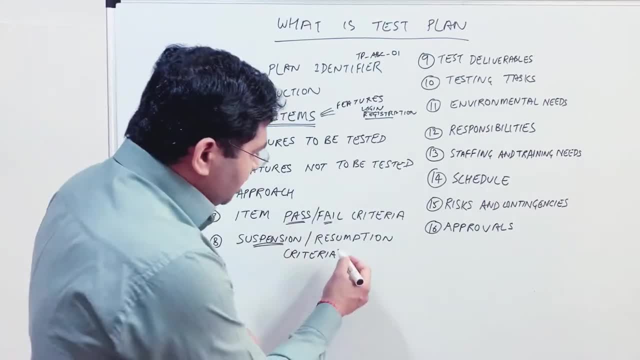 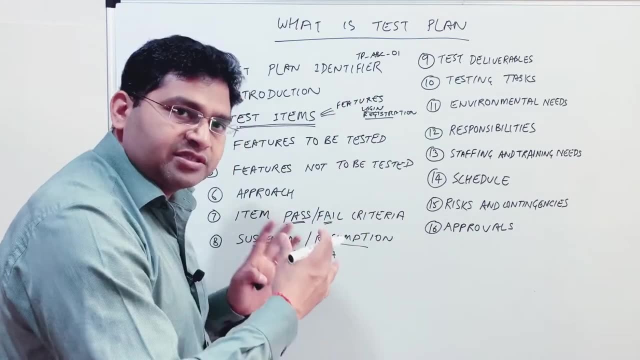 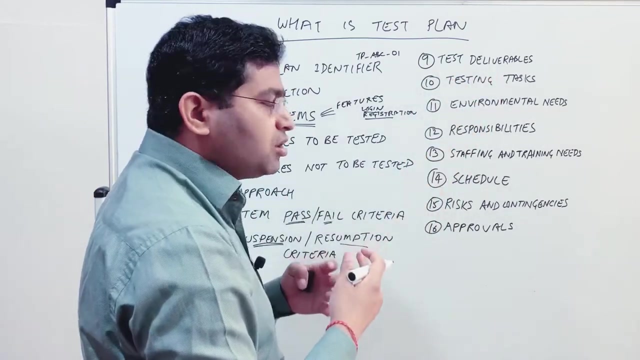 those defects will be fixed and verified successfully, we will resume our testing as per plan. right? so all those things will go into suspension and resumption criteria. okay, so these are the eight sections, now coming to the ninth one. so this is test deliverable. so what will? 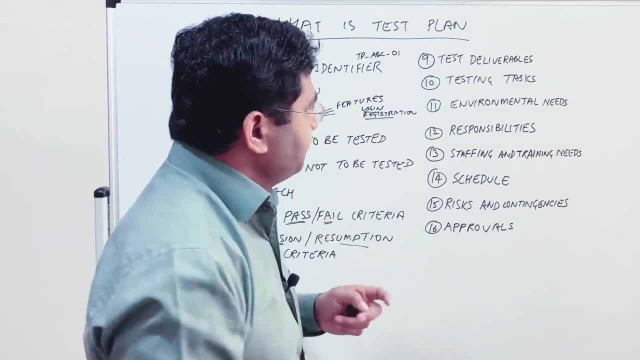 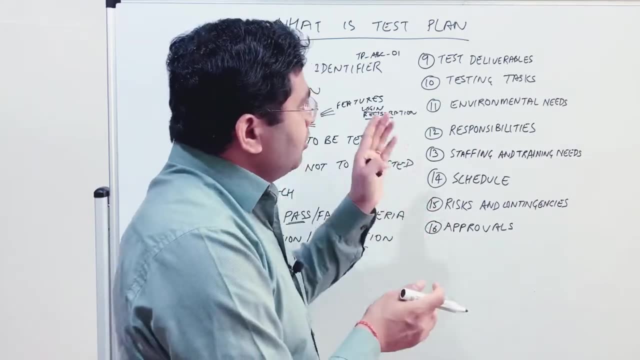 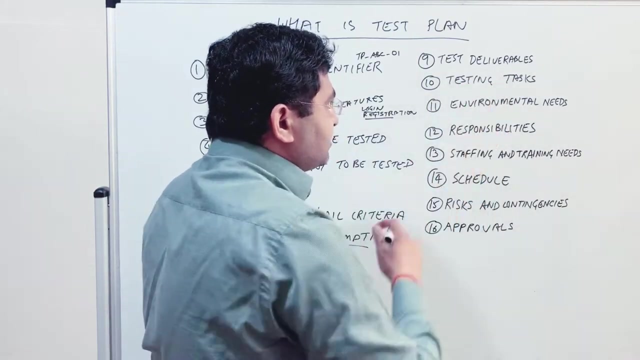 you will deliver as part of the testing. so you will deliver test cases, scripts, plan um. if there are any automation scripts that you are doing, all those deliverables, whatever deliverable has been agreed, you deliver or you mention that as the test deliverables. okay, then you have the testing tasks. 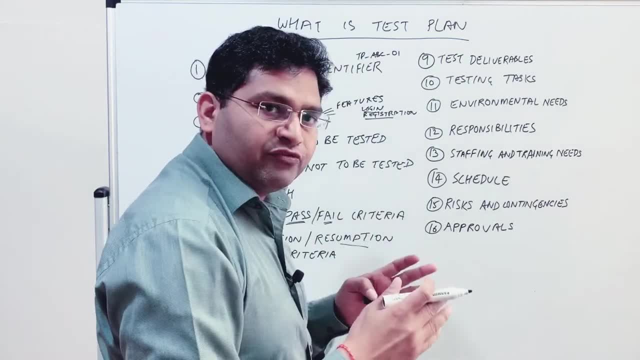 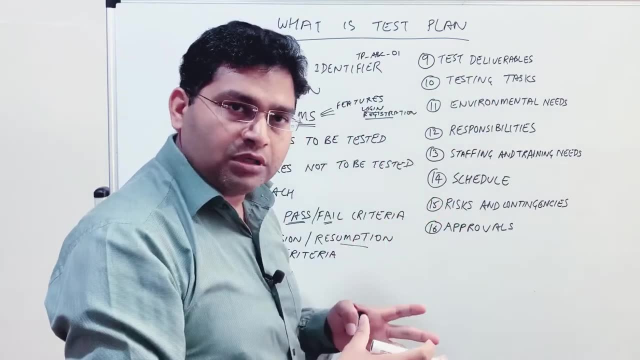 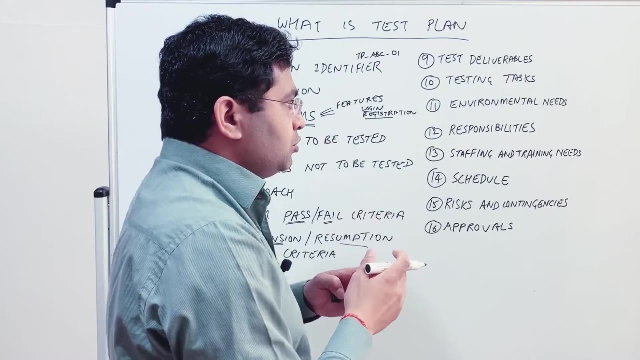 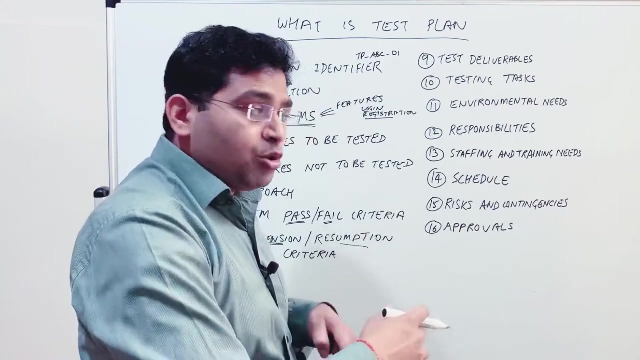 what all tasks will be required to perform all the activities. so what all testing tasks will be involved in the overall testing lifecycle, then in the environmental needs. what is the environment? so you know, Windows Server is required. you need to install something. what software version? what hardware version? how many? 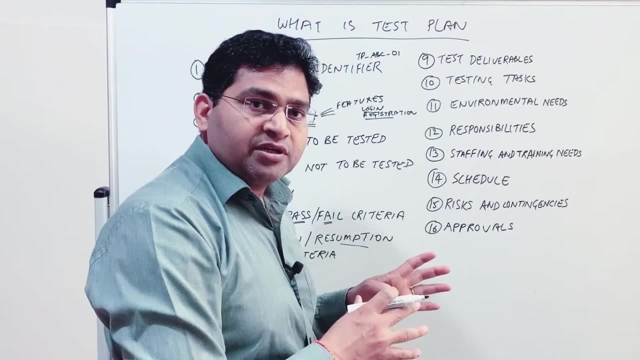 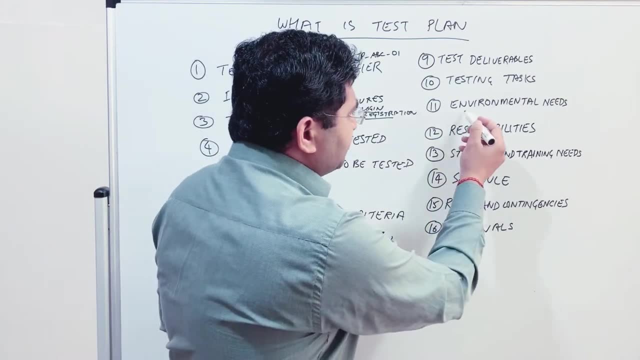 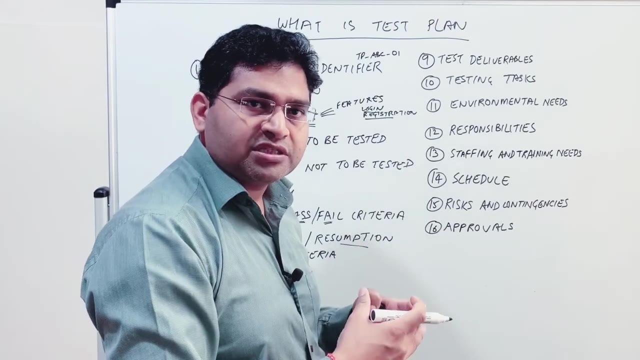 OS is required. if there is any tool specific, a specific tool required, any automation tool required. what test management? you know tools, so any any specific you know test environment related needs that need to be available before you can actually start. you know testing needs to go into environmental. 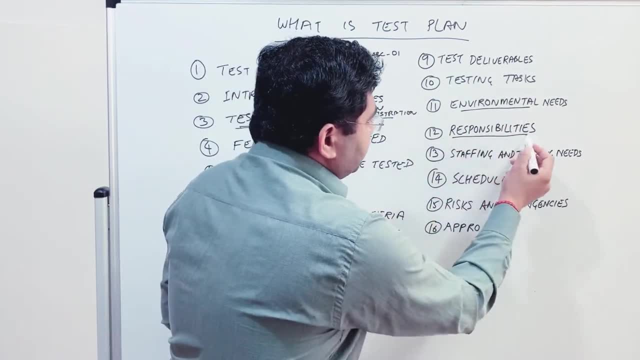 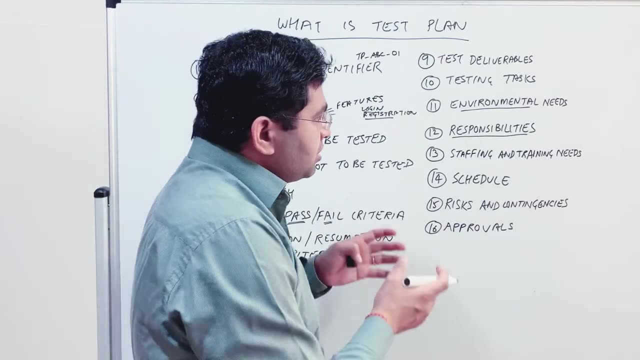 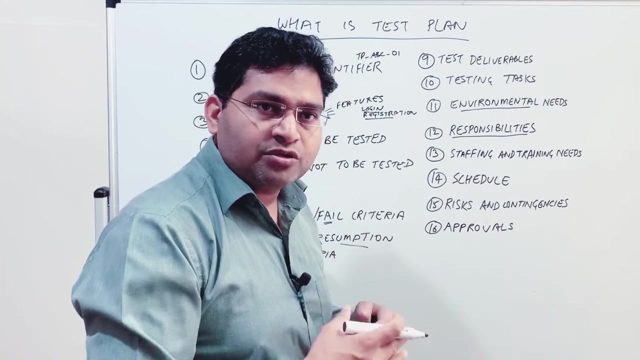 needs section? then in the responsibilities section, who is responsible for what within the team? right, so what test manager will do what test lead will do what a person within a particular testing team say, for example, I am the you know API tester or person who has expertise in the API testing? 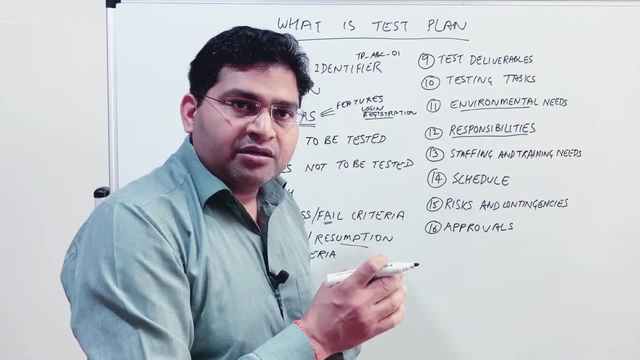 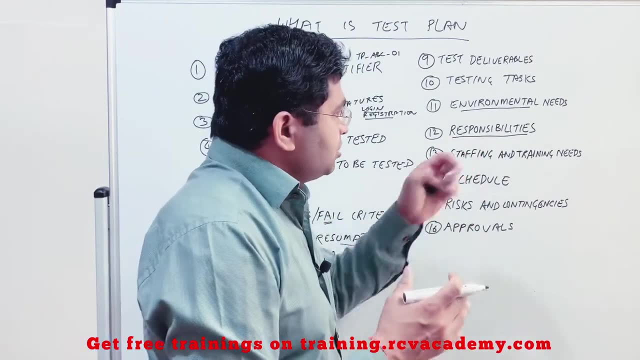 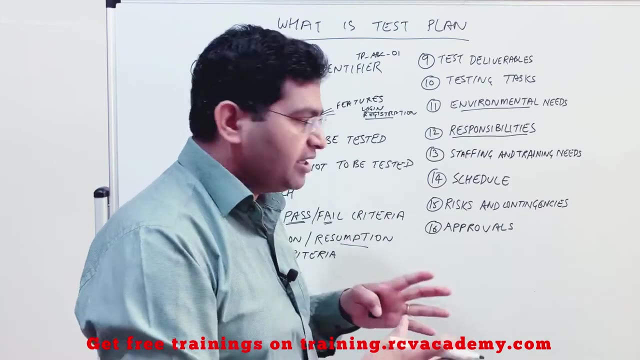 so I will be focusing more on the API related story. so any responsibilities or specific responsibilities that need to be defined will go into the responsibilities section. so test manager, test lead any team member, what all responsibilities are there for each of the team member will go into the 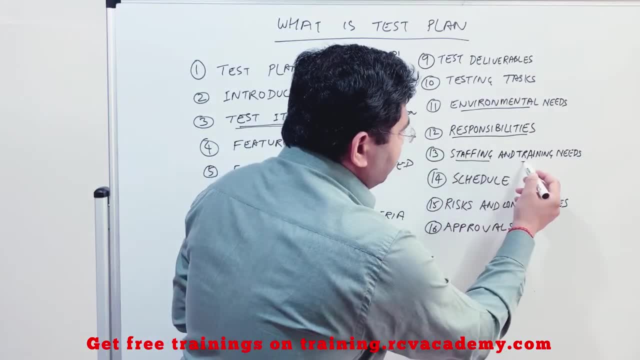 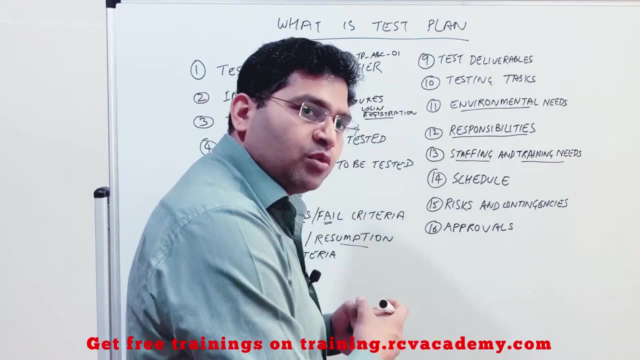 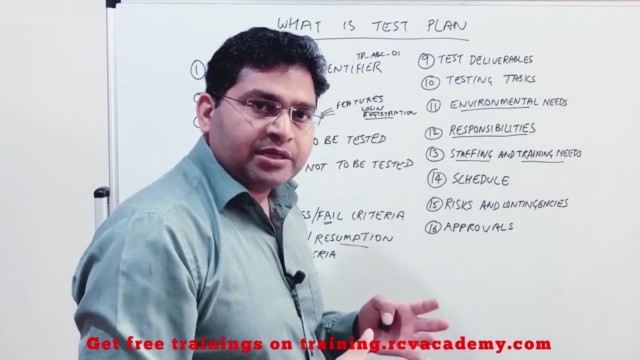 responsibilities section, then if there are any staffing and training needs required, then you will basically mention that in to the staffing and training needs. many people are required to basically achieve this particular project or finish the testing. if there are any training needs, say for example, i am going to use the new tool or new test. 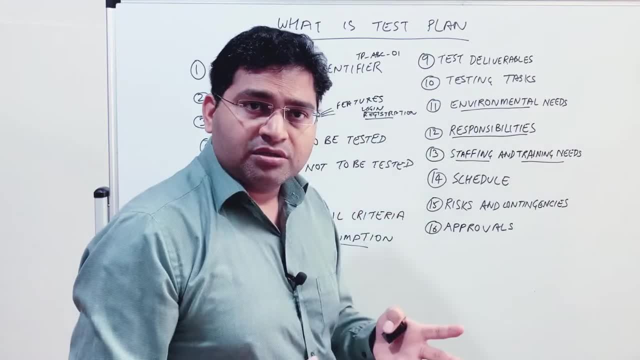 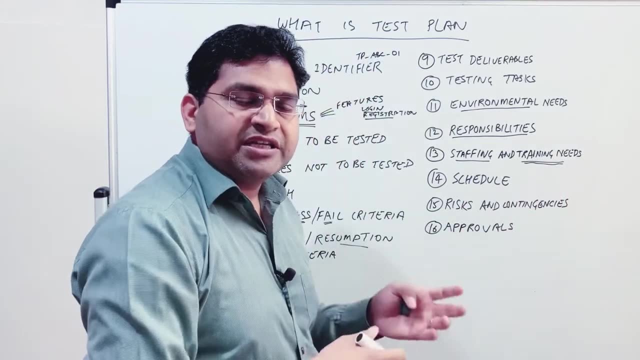 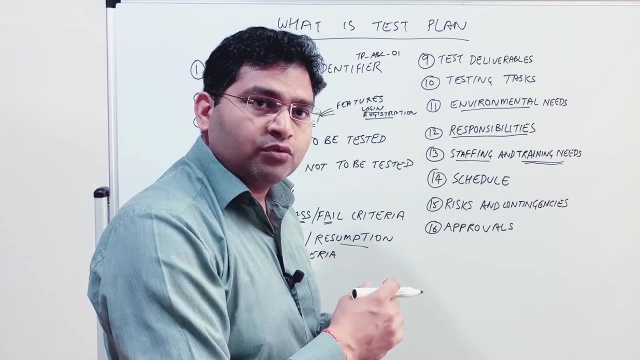 management tool for which the team is not a team is fairly new for it, then we'll have a brief training session for it. if there is any automation tool that is required, we can have training session for that. how many people will be required to perform that? overall testing will go into the 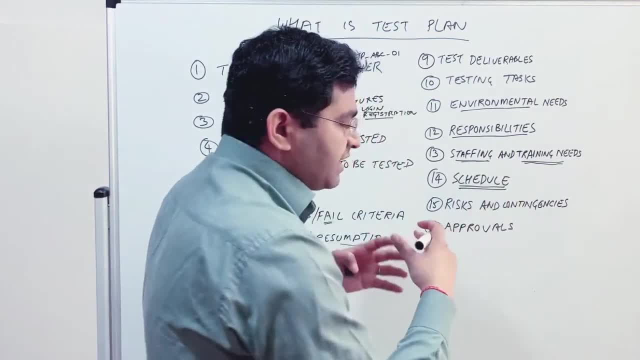 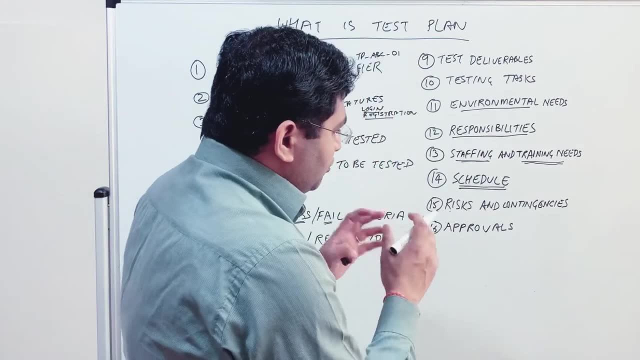 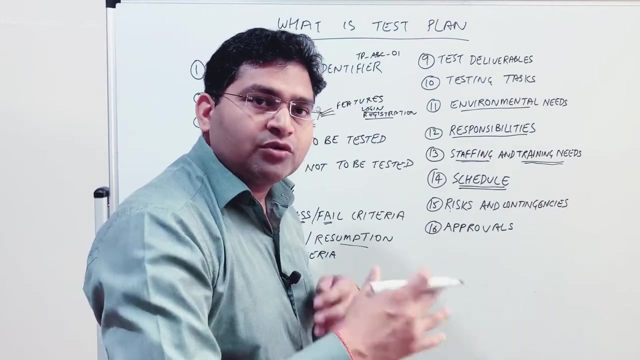 staffing section. schedule is basically, you know, like the timeline of the overall test activity will go into the schedule. then any risk and contingencies will go into the risk and contingencies section. in risks you mentioned, say, for example, what will happen if something goes wrong, wrong within the test life cycle. say, for example, you know team members get sick, is there? 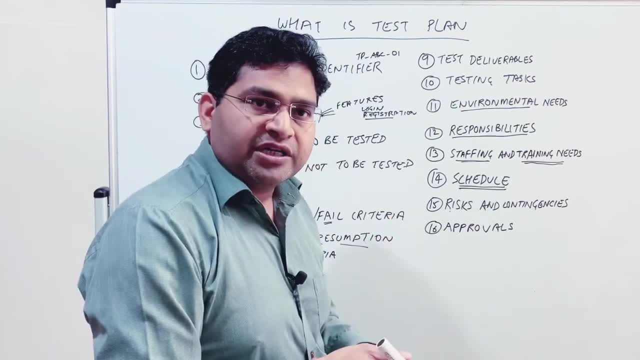 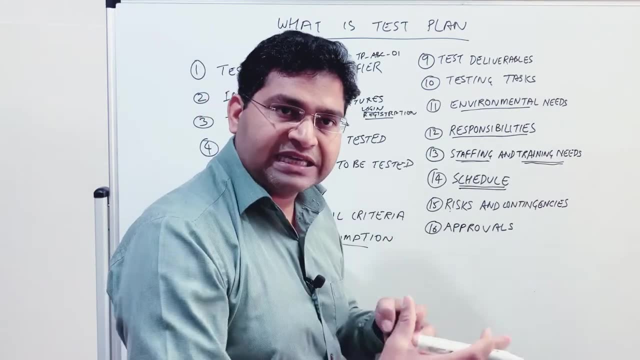 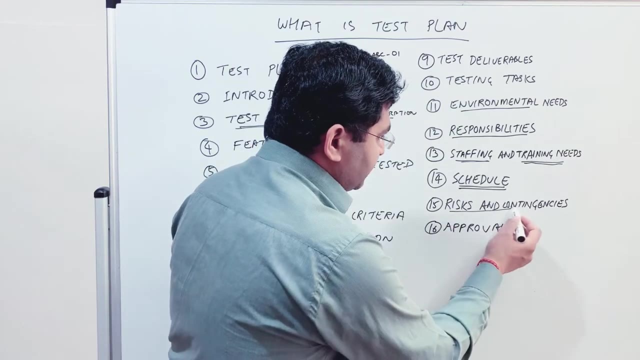 any contingency plan for that. if there is a blocker defect that has, you know, stopped or you know suspended our testing for three days, what all risks are possible in the overall testing life cycle will go into the risk and contingency section right, and then approvals will have the 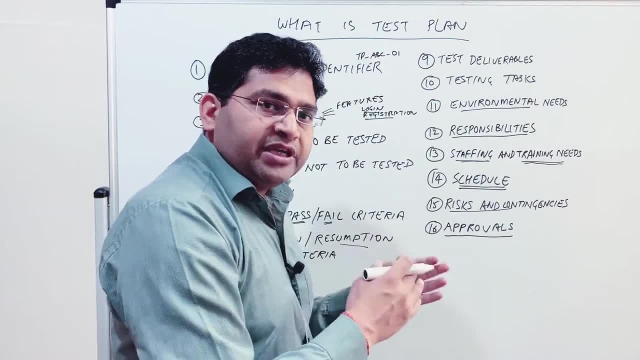 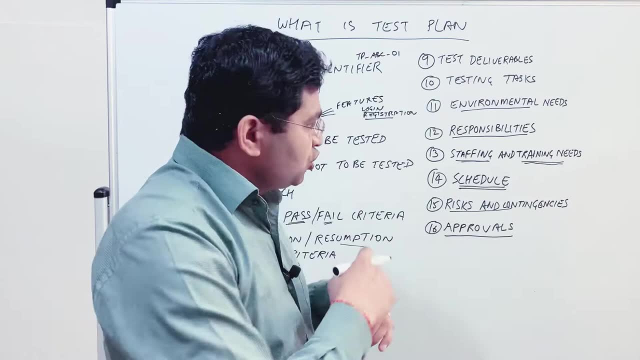 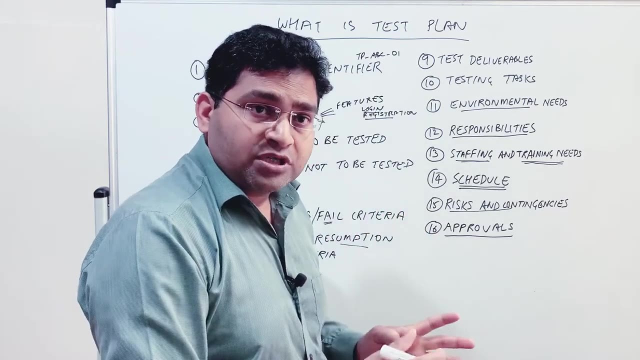 name of the approvers who will be approving this overall plan. okay, so, project manager, test manager, mostly, this plan, test plan is, you know, written by either by test manager or test lead, with the input from the overall team, if the team is there otherwise, from the experience of that, but you 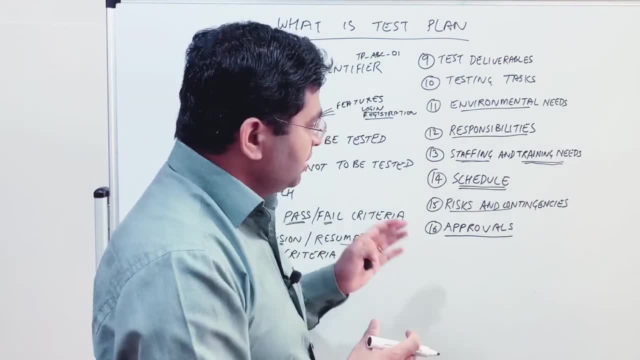 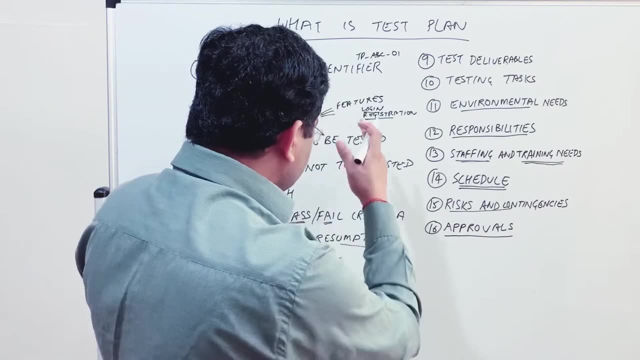 know a particular person, whosoever is test lead and test manager, and then they will be providing the details of all the people who are going to be approved for the test, and then they will be to approve this plan, right? so whatever has been documented in this plan like this is what we are. 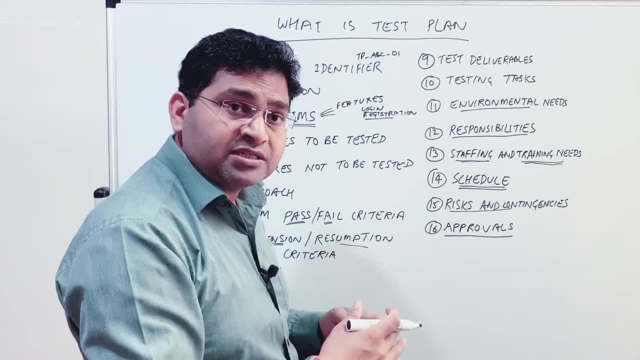 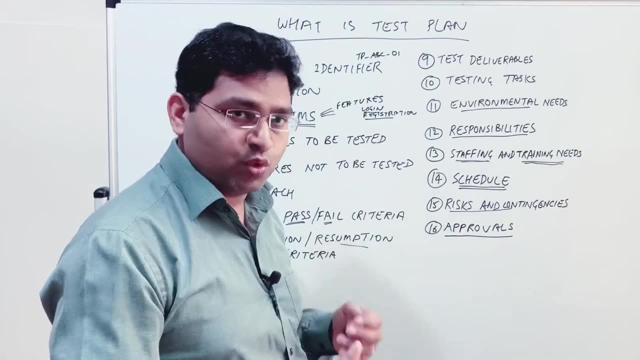 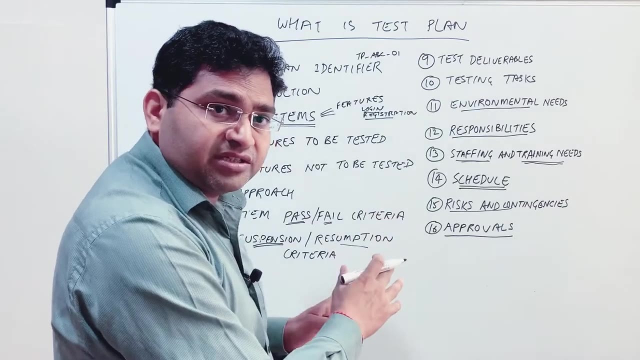 going to test. these are the features. this is how we are going to test who is going to test, this is the schedule, how it looks like, and these are the dates when we'll finish our work right. so this is. these are the key sections, or key 16- 16 sections as per IEEE. you know, test plan template, which will 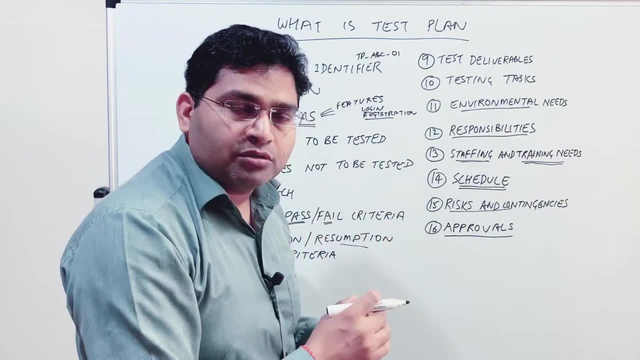 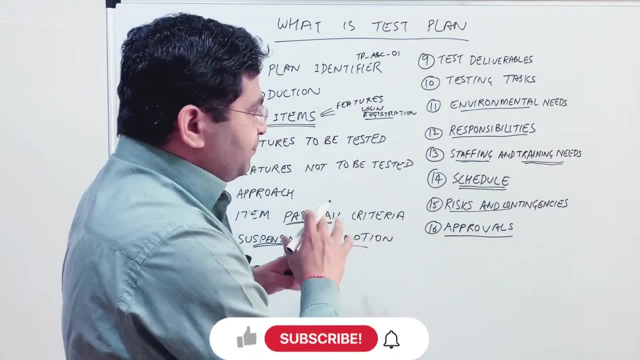 you know, be approved for the test plan, right? so whatever has been documented in this plan is going to be found in any test plan that you pick. so it will be. you know, it doesn't matter which organization you go, you will find these sections in every place there might be, you know. 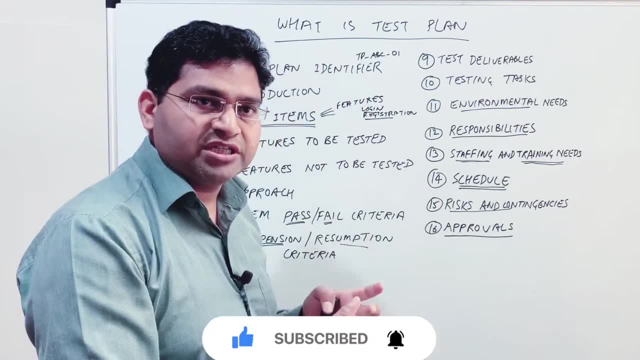 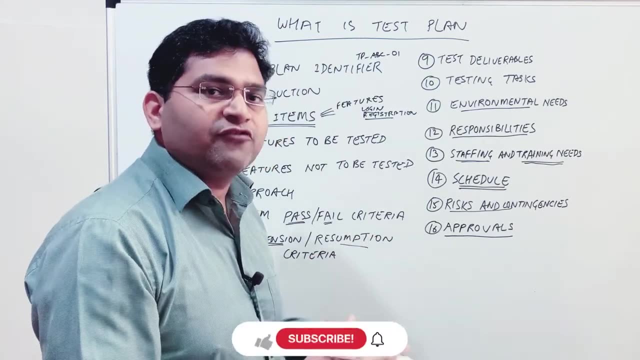 a difference in, you know, naming convention or the terminology that they use, but these sections will definitely be there, along with some more sections if it is relevant for that particular project or specific to that project, right? so these are some of the key sections that will be found in any test plan. 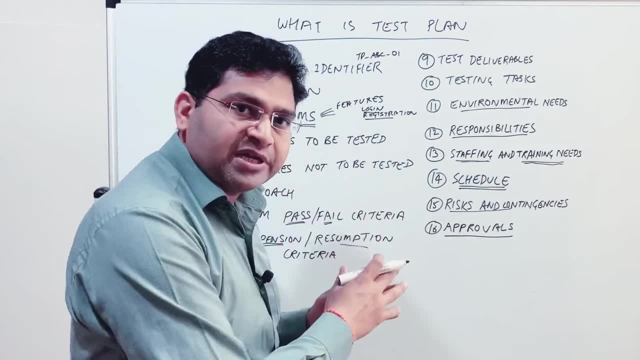 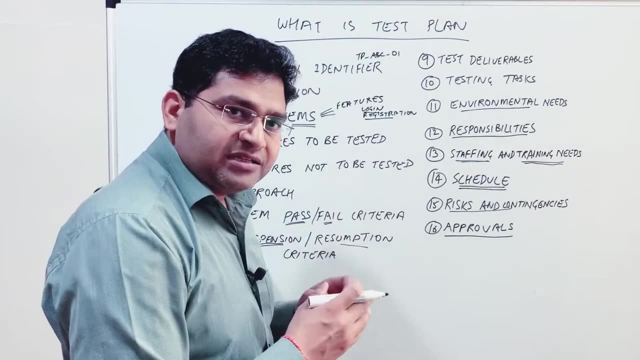 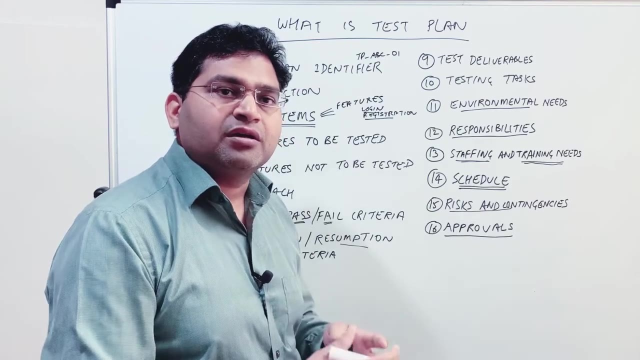 the you know these are, you know, key sections of a test plan that will be there and should be there in any of the test plan and test plan. once you write this, it will guide your thought process how you are going to approach the testing for a particular project or application, right same. 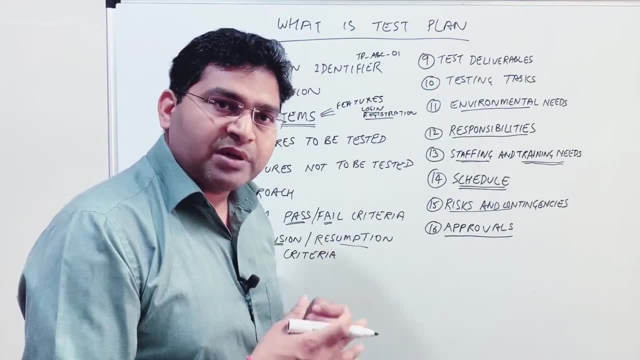 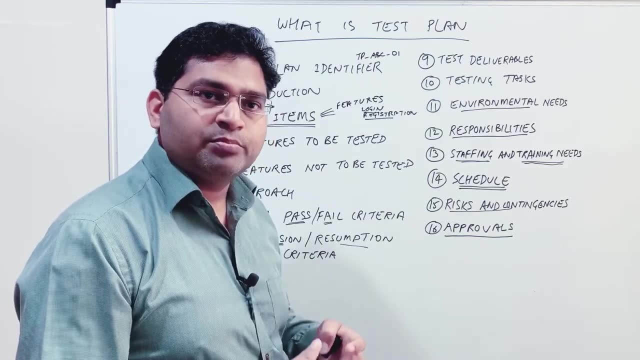 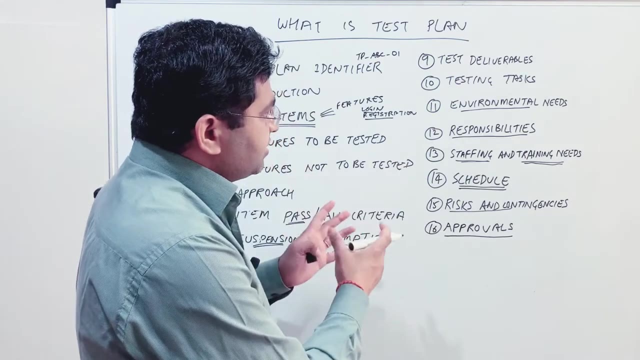 analogy as building the house. if you do not have the plan and you haven't thought about how you are going to perform plumbing, or how you are going to perform plumbing or how you are going to perform plumbing or electrical work prior to building the rooms and roof, then you know in software testing. 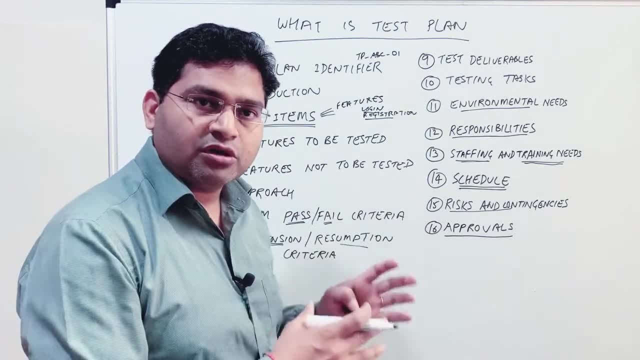 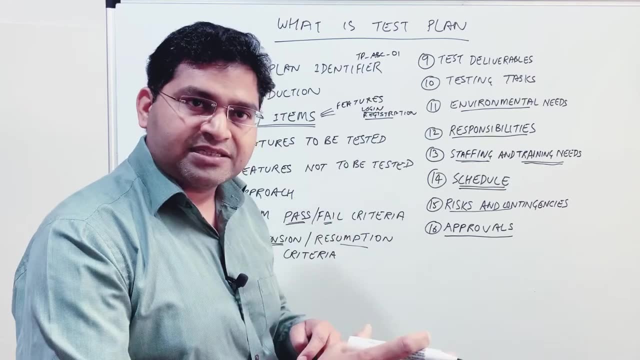 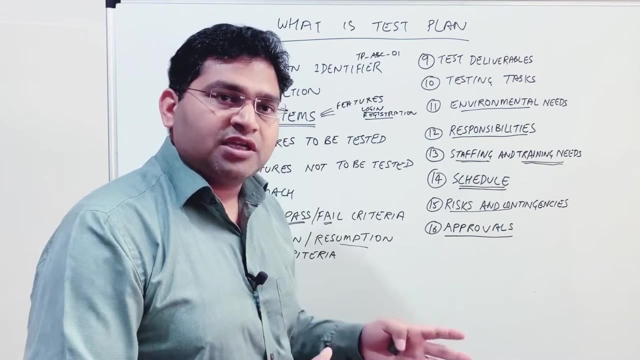 term. it's similar. so you have to, you know, give a thought up front to basically how you are going to lay your foundations, how you are going to approach testing to that particular application, what all is required, how many people are required, what will be the timeline to deliver that particular you. 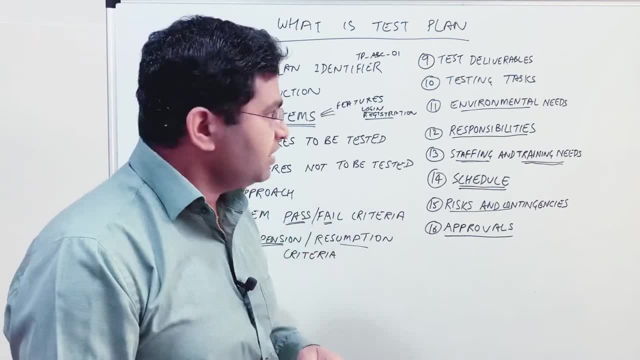 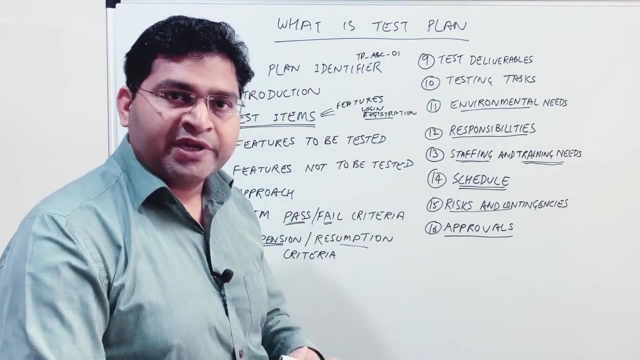 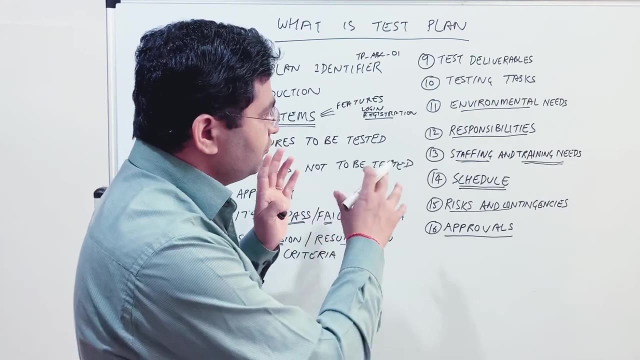 know testing for that particular application or software. okay, so that is all about. you know a test plan and what exactly is a test plan now going through? you know any of the you know Google templates. you can find there are few things here and there are. you know few sections renamed differently. that doesn't make difference. these: 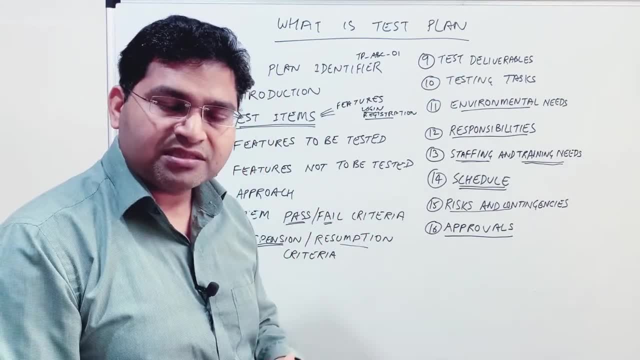 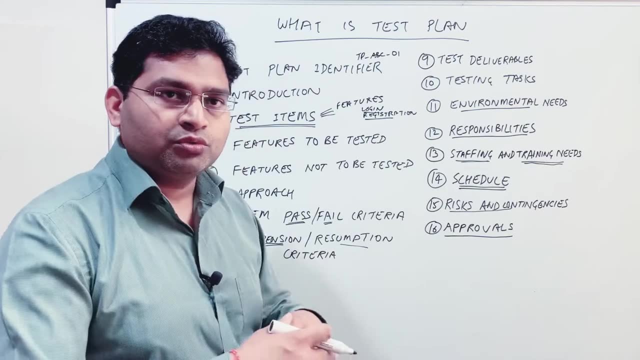 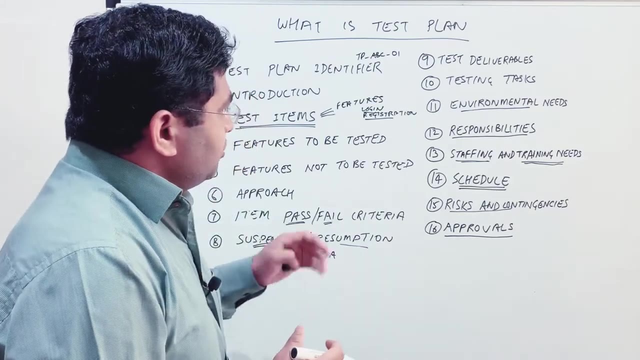 are the key sections that you can correlate with any of the plans, test plans available out there and you can also- you know you, you might also find some new sections. so you, if new sections are available there, they might be specific to the projects. okay, so this is all about the test plan: why you need a test plan and how it helps you to. 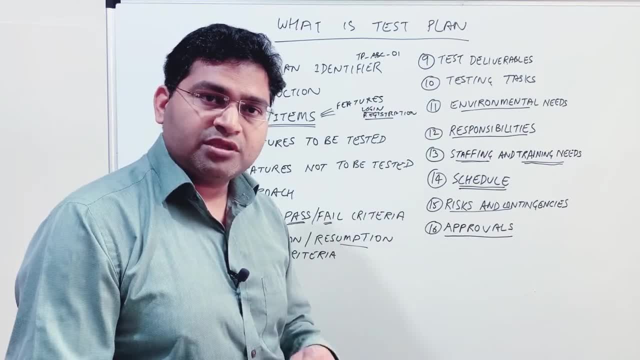 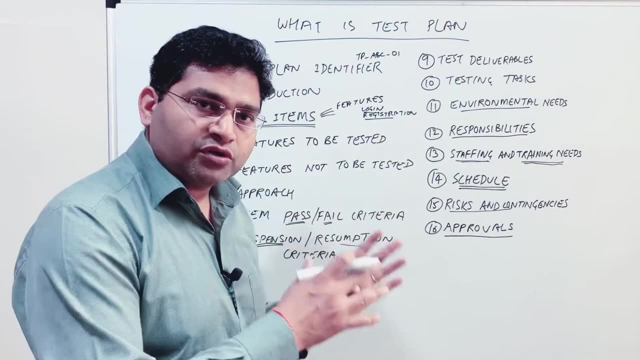 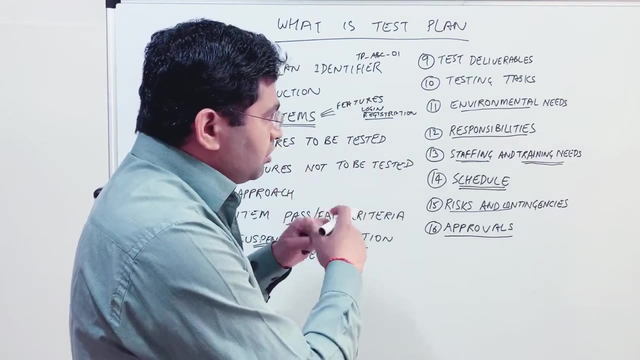 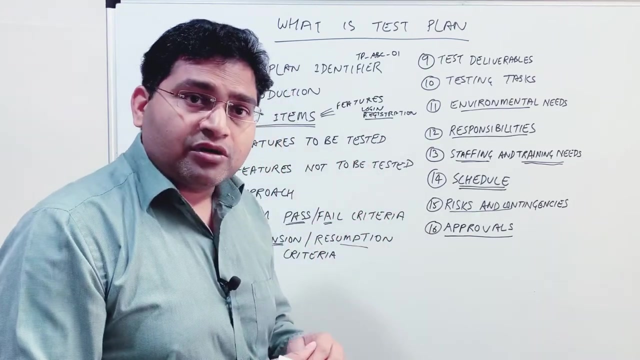 basically perform the software testing with proper approach and confidence. now, this is- this was more relevant with the waterfall approach and still even with agile approach. these are the things that you know are quick test planning is done and required, but it is not as detailed or it is not a phased.